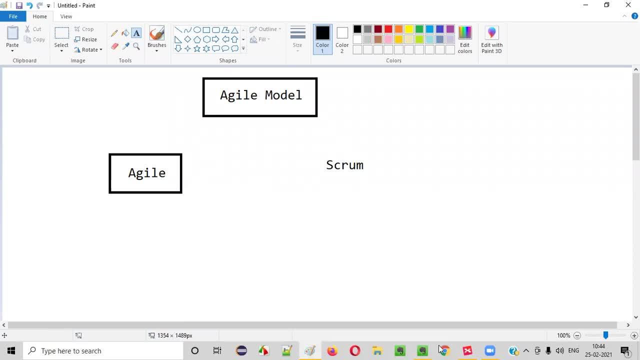 Is Scrum equal to Agile? Scrum is not equal to Agile, guys. Agile is a different term and Scrum is a different term. Everyone thinks that Agile means Scrum. That is a problem, guys. They are not the same. 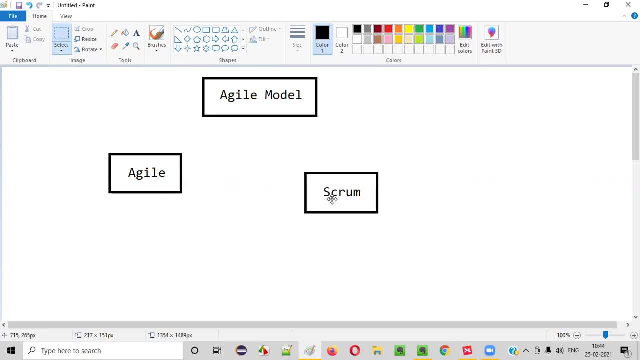 But what is Scrum then? How is Scrum related? How is Scrum related to Agile? Scrum is one of the methodology guys. Agile has a lot of methodologies. Scrum is one of them. Other methodology we have under Agile is along with Scrum. under Agile we have different methodologies that can be followed in the projects. 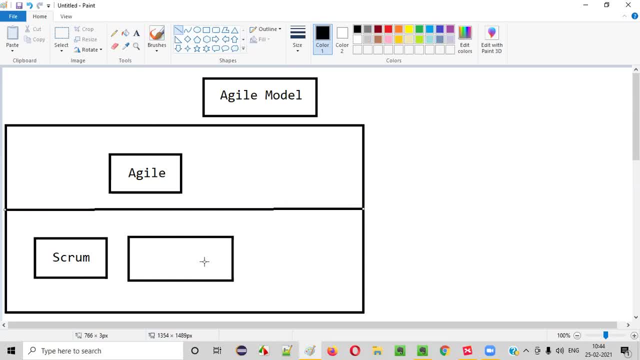 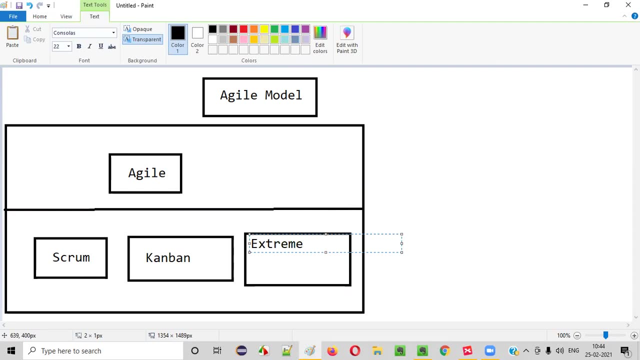 You can apply either Scrum methodology to the project as part of Agile or you can apply Kanban. There is something like Kanban, Something like Extreme Programming. A lot of things are there, guys. okay, A lot of things are there. A lot of methodologies are there, Extreme Programming And many more are there. 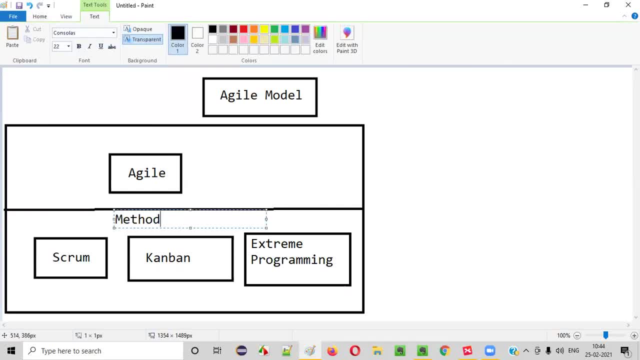 These are all methodologies, guys. Scrum is an Agile methodology. It's not Agile, guys. Scrum is not Agile. Scrum is an Agile methodology. okay, So fine, If you come here and expand this Agile, you can see that. 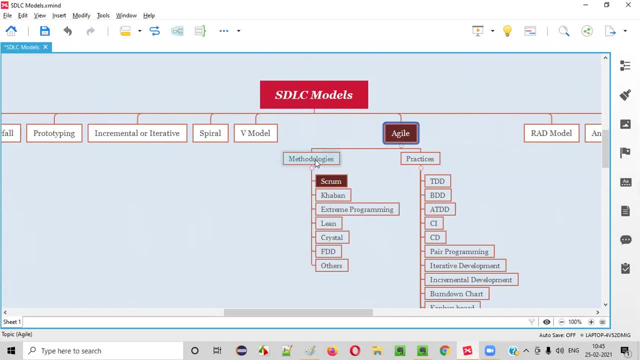 Agile has. okay, Agile SDLC model follows different methodologies. okay, We can follow different methodologies of Agile and we can follow different practices of Agile. Agile can be categorized or can be like explored more in terms of these methodologies and practices, guys. 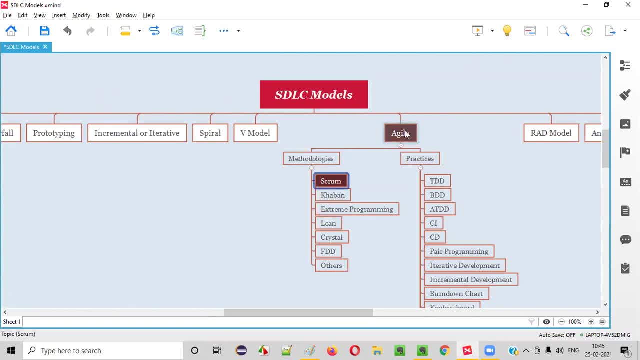 In terms of methodologies, Scrum is one of the Agile- okay, One of the Agile methodology guys. Scrum is not Agile guys. Scrum is an Agile methodology. Panda is not Agile. Come up with better industrial methodologies, okay, And we can say Agile HDLC guys. You can see the Commun enjoy with hard adoptations. you can say, well, we should use the microphone because it's easier to generate audio from there. 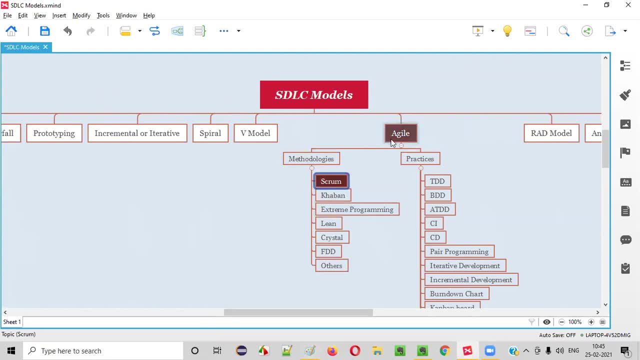 Okay, one of the Agile methodology guys. Scrum is not Agile guys. Scrum is an Agile methodology. Okay, it is a part, guys. It is a part of Agile, not complete Agile. Everyone thinks Scrum is Agile because in all the projects, guys. 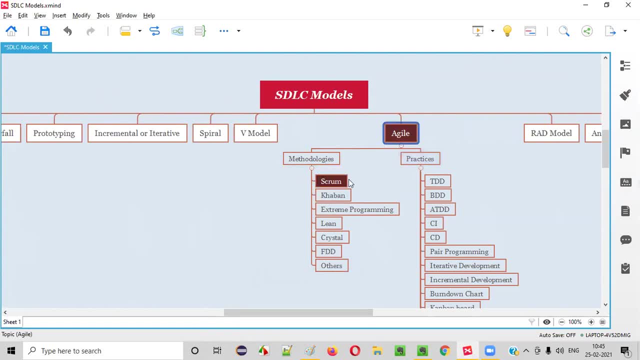 in most of the projects, everyone is using this Scrum methodology of Agile. That's why people think that Scrum is Agile. That's not correct. Okay, Scrum is part of Agile, Along with Scrum in Agile. there are other methodologies also. 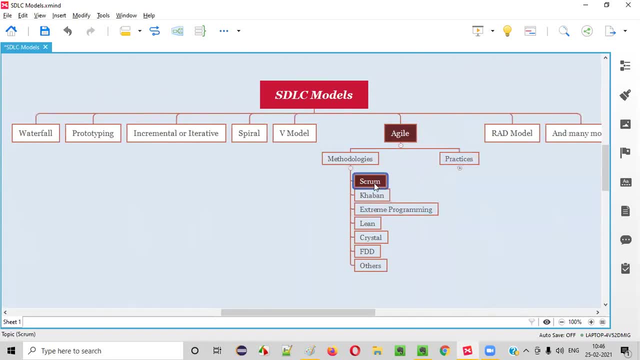 What are they? Okay, along with Scrum methodology of Agile, there are other methodologies in this Agile. What are the different other methodologies of this Agile Apart from Scrum? we have Kanban, Okay, then we have Extreme Programming, Then we have Lean methodology. 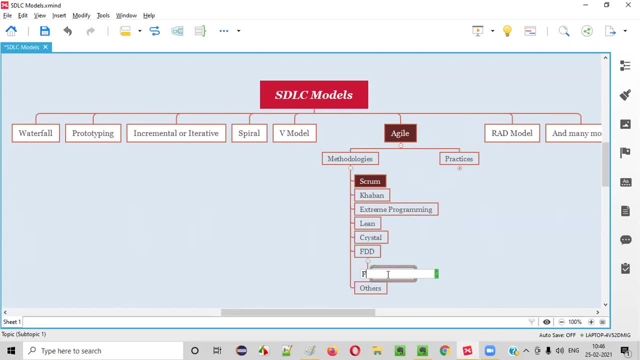 Then we have Crystal methodology. FDD stands for Future Driven Development, guys. Okay, this is another methodology. okay, Future Driven Development methodology. And there are many more guys. There are many more methodologies under Agile. So Scrum is what guys. 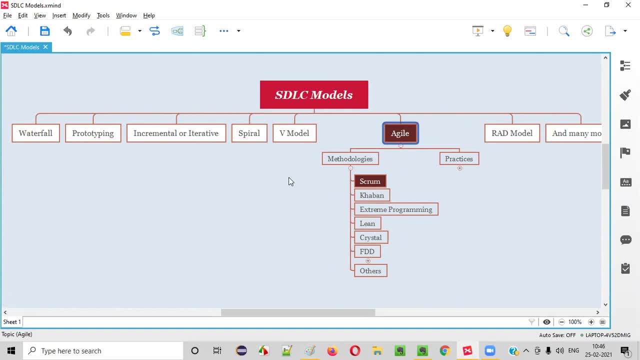 Scrum is one of the methodology of Agile. okay, When someone asks you about Agile, don't explain about Scrum. guys, Explain like this: Agile has several methodologies and practices. Scrum is one of the methodology of Agile. Then you can explain about Scrum if you want, okay. 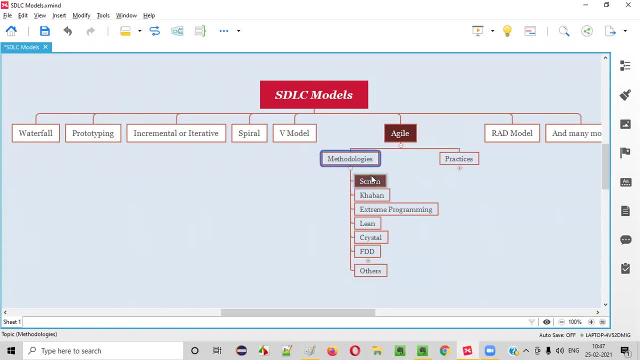 But don't directly start with Scrum and explain. That is a mistake that everyone makes because of this small confusion. But what about this? Scrum is one of the best practices, guys. okay, Scrum is now a methodology of Agile. 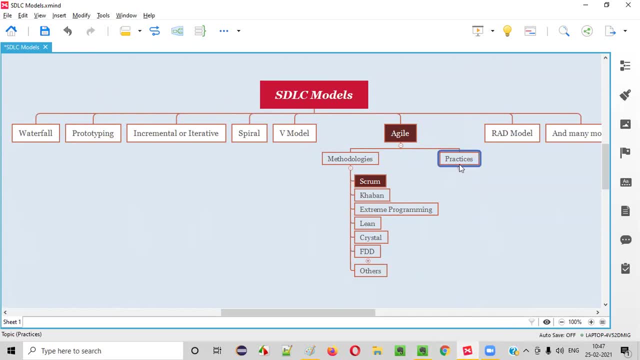 That's fine, But what about these practices? Practices are nothing but the best practices, guys. It's like add-ons. okay, When you are following the Scrum methodology in Agile as an add-on? okay, as an extra add-on. 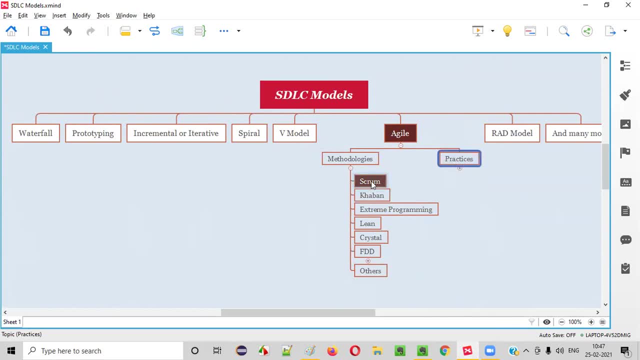 you can follow any of these best practices. okay. Scrum plays some best practice. Kanban plays some best practices. Extreme Programming plays some best practice. Like that you can follow, guys. Practices of Agile are nothing but the best practices, guys. 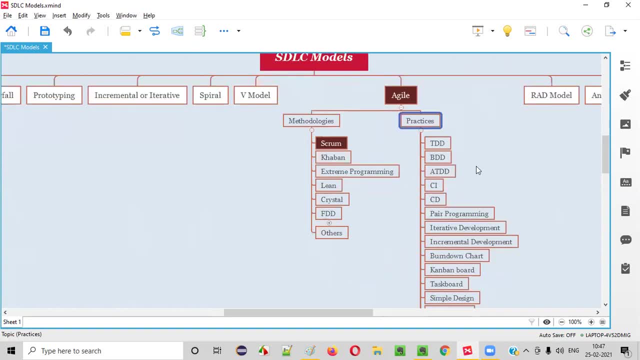 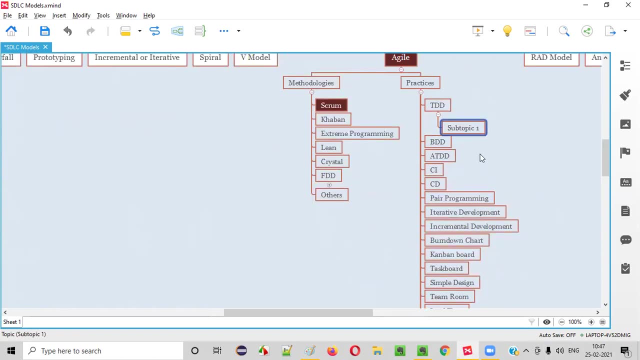 When I expand these practices, you can see there are a lot of several best practices in Agile guys. okay, Agile supports several best practices. One is TDD. TDD stands for Test Driven Development. okay, This is one of the best practices. 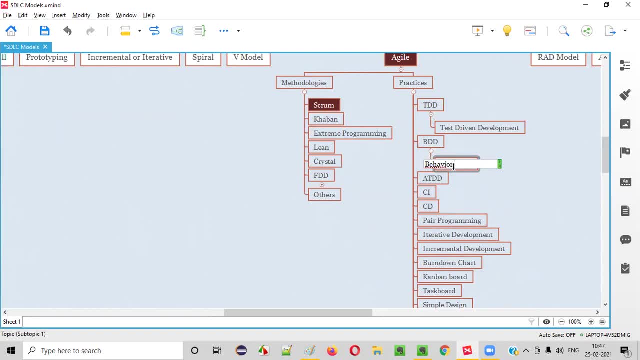 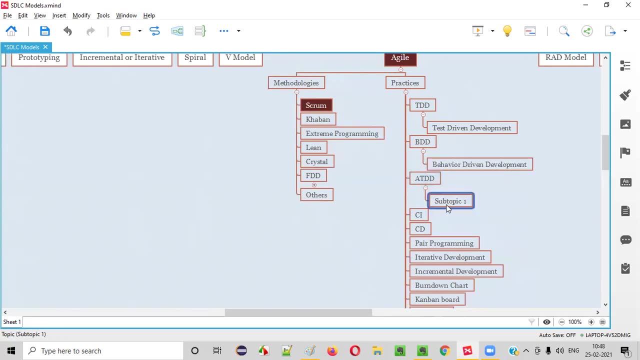 Then we have BDD- Behavior Driven Development. Then acceptance- This is acceptance: test-driven development. These are all the best practices of Agile guys. okay, Along with Scrum, you can use TDD. Along with Scrum, you can use BDD. 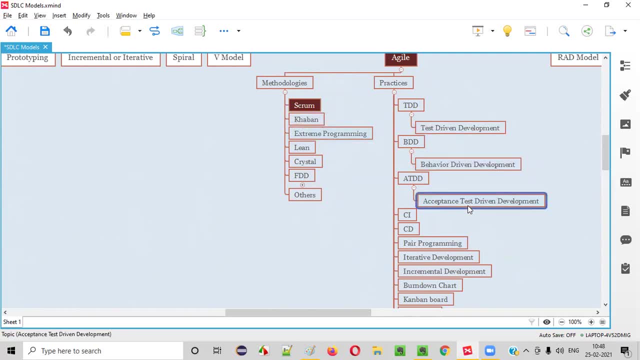 Like that: along with Kanban, you can use TDD. Along with Kanban, you can use BDD. Like that, guys, okay. These are add-ons, kind of best practices. CI is there, okay. CI stands for Continuous Integration, guys okay. 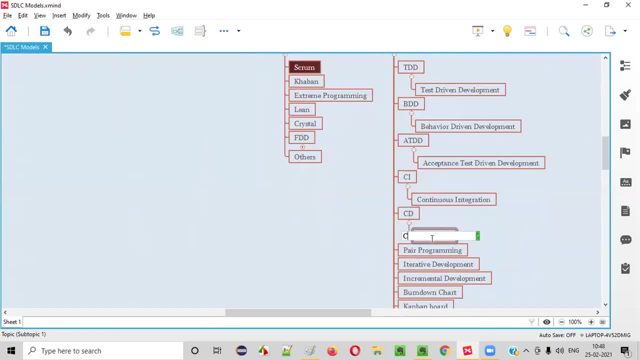 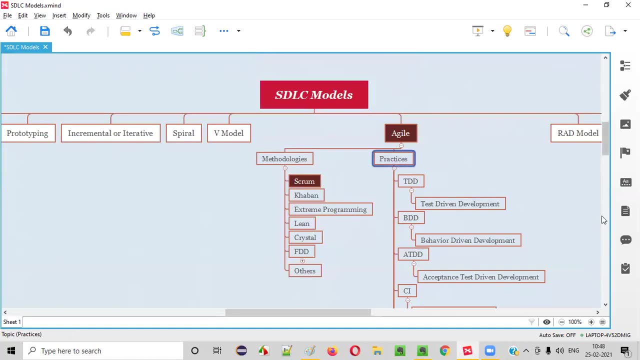 CI stands for Continuous Integration. Then we have CD- Continuous Delivery, Continuous Delivery. So what is the purpose of these best practices? When you apply these best practices, you will definitely get some benefits, guys. okay, Maybe the communication will become proper in case of applying this behavior-driven development. 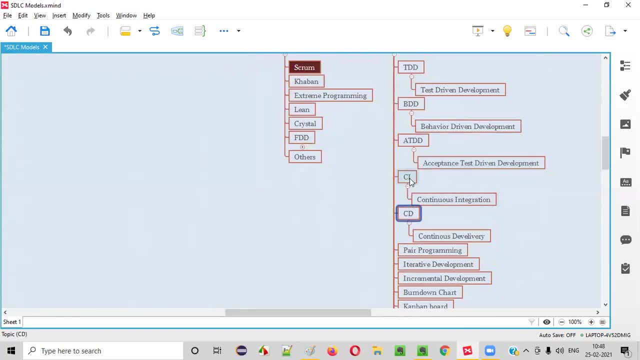 Or, if you go with this CI CD, the delivery cycle will become speed. okay, You can fastly deliver the things into the market. because of this, continuous integration and faster development will happen because of continuous delivery. The faster delivery will happen Like that. 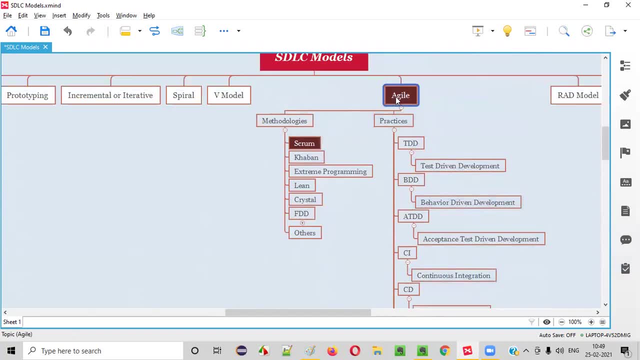 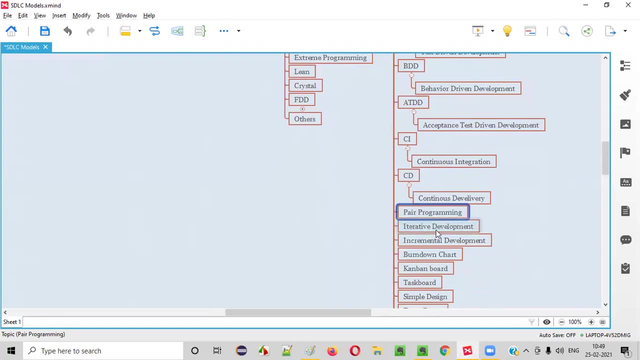 Each and every best practices, when followed by this agile in one of the projects has a purpose, guys. okay, That will benefit the project. Pair programming is there. Then we have iterative development. is there Incremental development- Burn-down chart: okay. 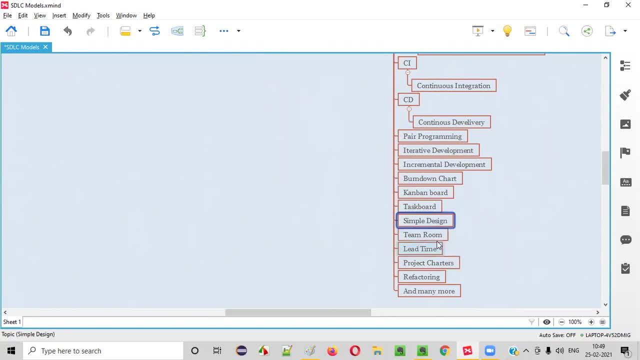 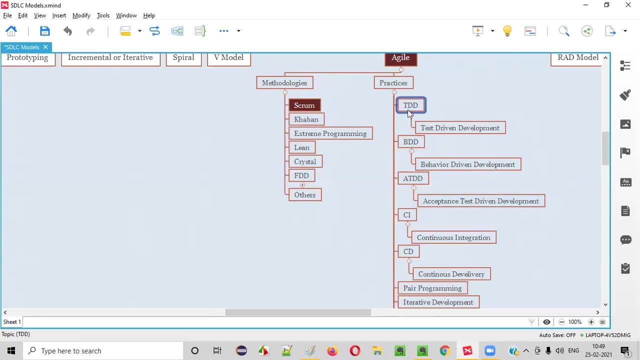 Then we have Kanban board, task board, simple design, team room, lead time. You don't have to remember all these things, guys. okay. The major ones that we generally see are TDD, BDD, TDD, BDD, CI, CD, okay. 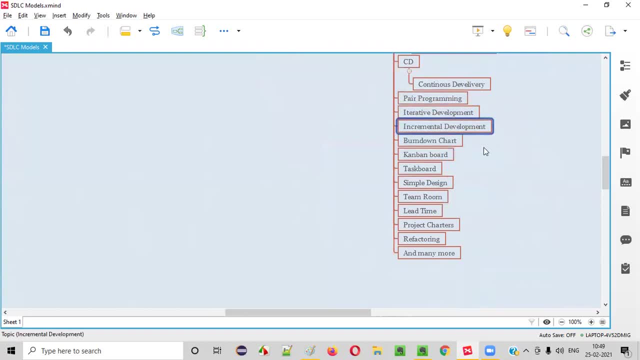 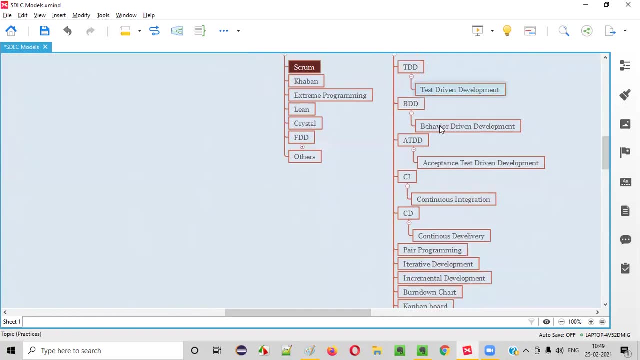 Okay, So these are like general words you can remember. okay, Iterative, incremental: you already know. So Kanban is something important. okay, Like that, few things are important, guys. You don't have to remember all the best practices here. 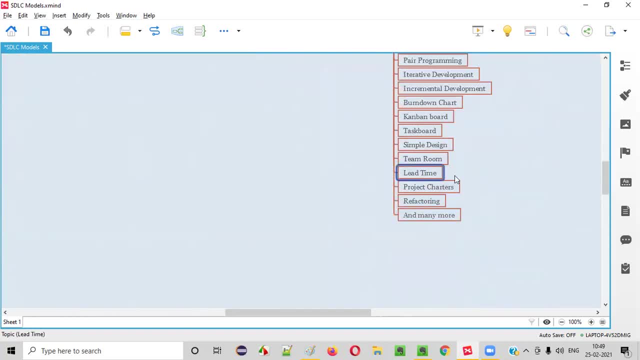 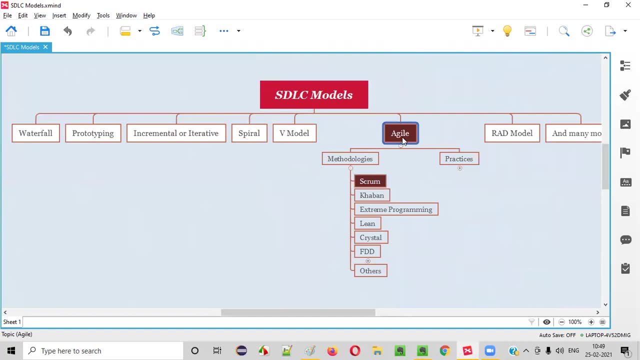 Few best practices you can remember, guys okay. Refactoring, project charters, lead time, team room- All these are best practices of agile, guys okay, Best practices of agile. So agile can be okay. If I have to explain agile in a detailed manner, I have to start saying that in agile, SDLC model. 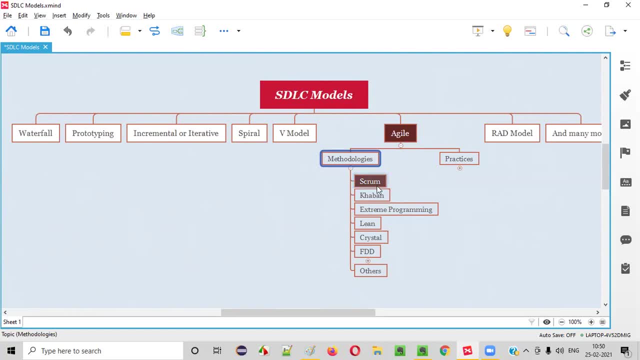 there are several methodologies and practices. Coming to the methodologies, apart from scrum, we have Kanban, Extreme Programming, Link, Crystal, FDD and many others Coming to the best practices that can be applied or practices of the agile. these are the practices. 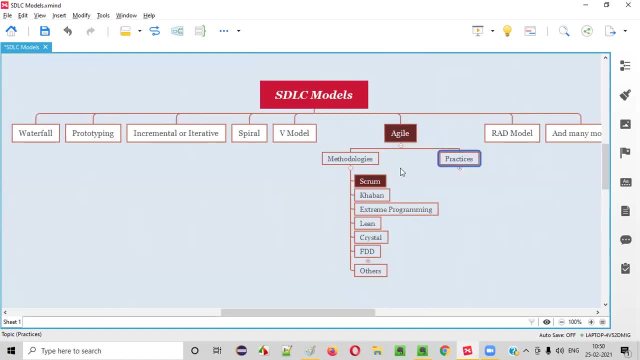 TDD, BDD, ATDD, CI, CD and so on. You can start explaining like that And after explaining about this thing then, so you don't have to explain all the more methodologies and all the practices, right? 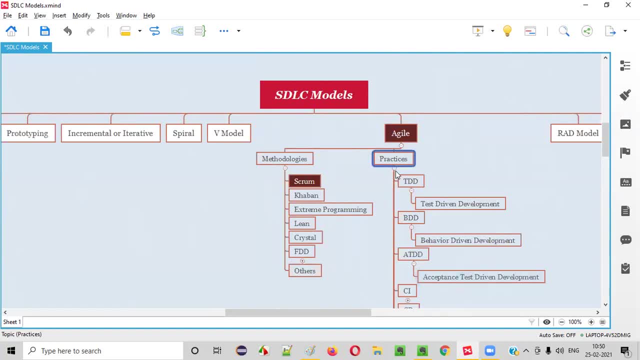 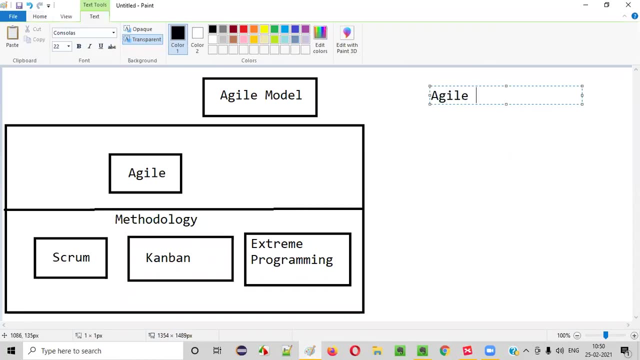 You don't have to explain each and every methodology here and each and every practice here. Rather, you can explain about scrum guys. okay, Saying that, let me explain, Okay, One of the- let me explain one of the agile scrum methodology. okay, 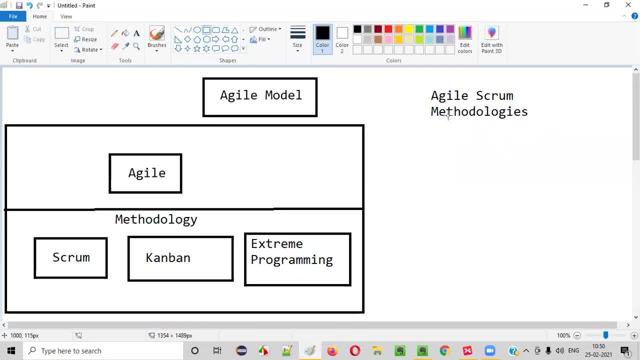 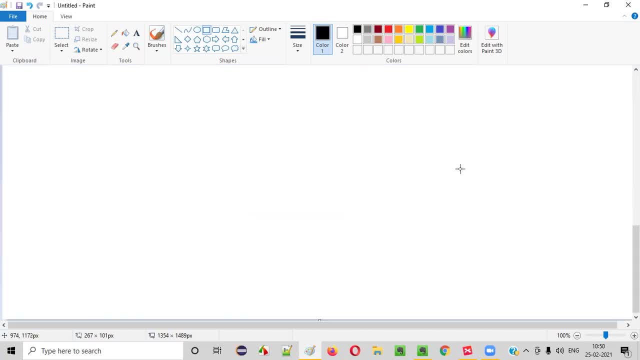 Though there are many methodologies available in agile, in the projects generally we follow scrum methodology. There you have to start and then start explaining about scrum. Then it's correct, guys. okay, Then we can start about scrum methodology. 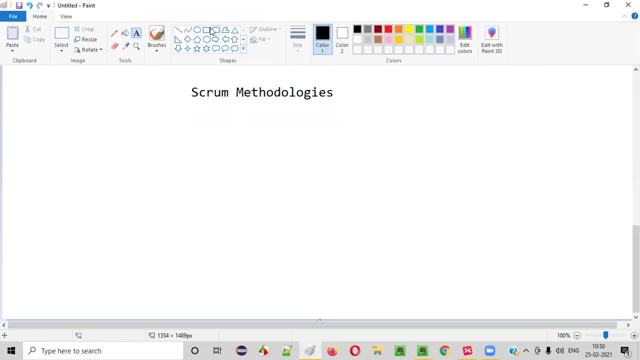 What is this scrum methodology? Anyhow, guys, anyhow, what I want to do here is: in this session, I will not be covering all the methods. I will be explaining all these methodologies and all these practices of this agile, okay. 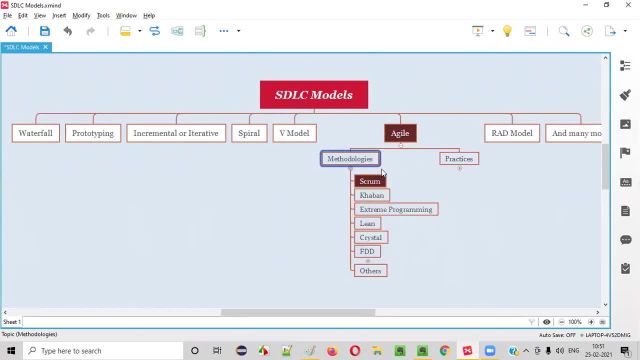 I will be explaining this agile at a high level, And I will be explaining only this famous methodology of agile, that is, scrum methodology. But in the coming sessions- okay, the coming sessions- what I will do is I will take this: 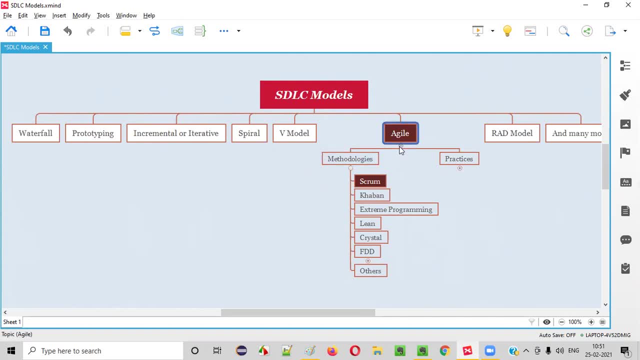 agile as a separate, okay Separately. I will try to explain agile guys in the coming sessions or something. I will explain agile in a separate or detailed manner where I will be covering each and everything about agile guys, okay. 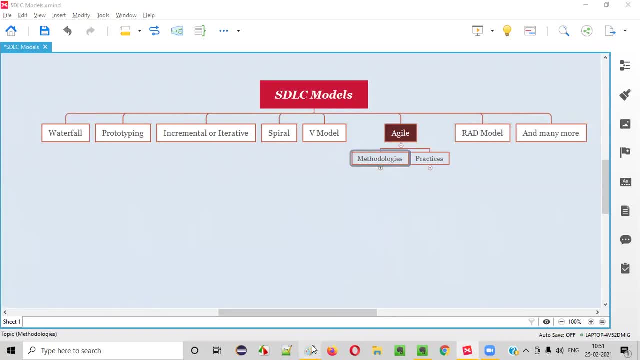 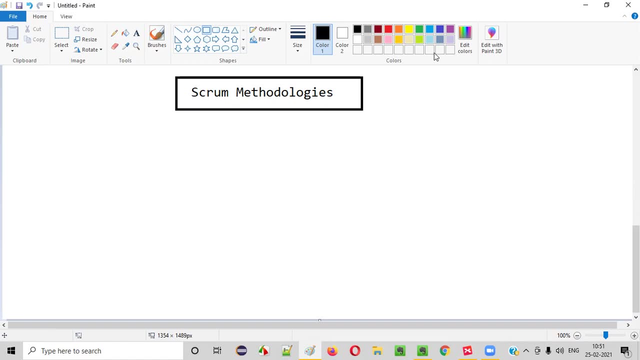 For now, this will be enough. okay, For this video. This is enough. So what are these scrum methodologies we have? What is this scrum methodology actually? okay, Let me explain this. One of the methodology of this agile SGLC model that is scrum methodology. 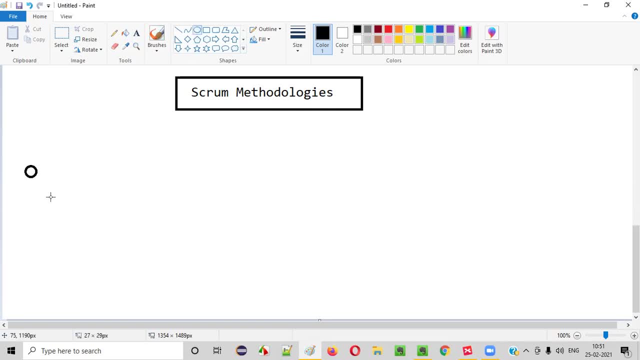 As part of this scrum methodology. what will happen? Let me explain. It all starts with the product owner guys. okay, There will be someone known as product owner, okay, So who knows complete business and all the stuff? right? 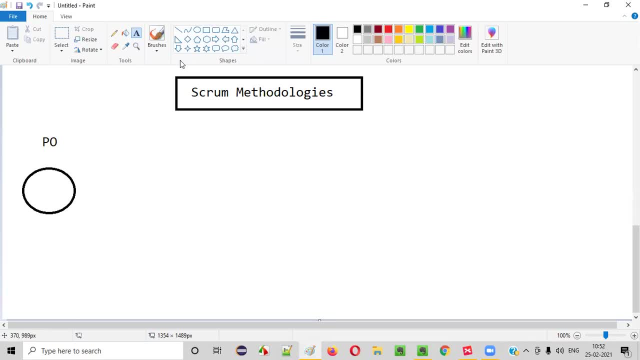 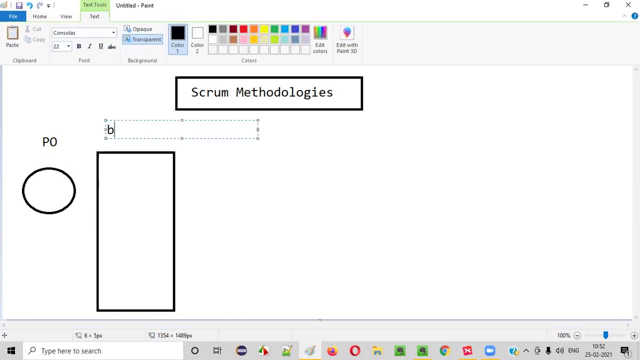 What this product owner does at the beginning of the project is he will actually create a bucket, guys. okay, There will be a bucket In this scrum. there will be a bucket. There's something like bucket. Let's assume that this is bucket, okay. 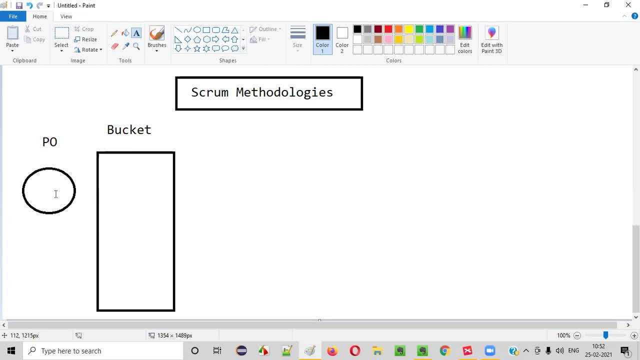 This product owner, who has knowledge about the application, complete knowledge about the application and business of the application, right. What he does is he will break the requirements of the software to be developed. He will break that requirements into small chunks like this: 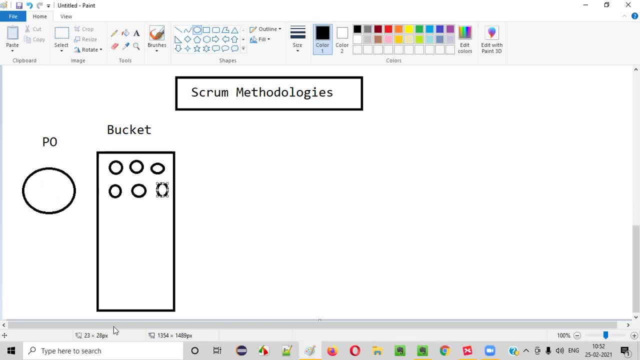 He'll break the requirements into small chunks, Instead of this Single document having all the requirements. he will break the requirements of the software required, developed the software that need to be developed into smaller chunks like this, guys, okay. Smaller pieces, dividable pieces, he will create okay. 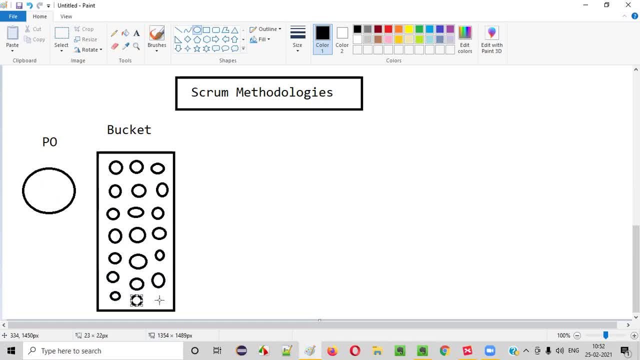 These are small chunks, So generally we call these smaller chunks of these requirements. okay, Each and every piece has a requirement, some requirement related to the required software. So all this together will become the complete requirements. These are the requirements of the software to be developed, kind of okay. 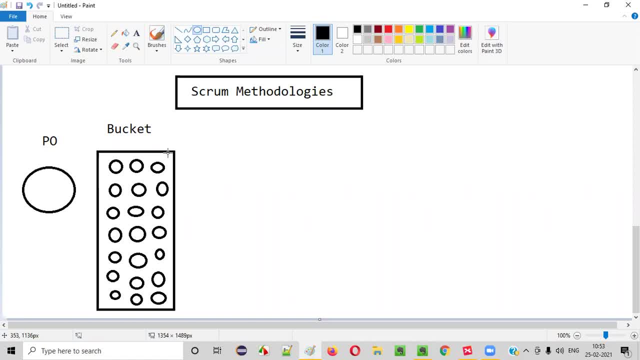 These are the requirements for developing. the software are divided into smaller chunks, like this They are generally known as the terminology for them is user stories. guys, okay, We call them stories, user stories, we call them. okay. So the requirements broken into smaller chunks and put into the bucket by the product owner. 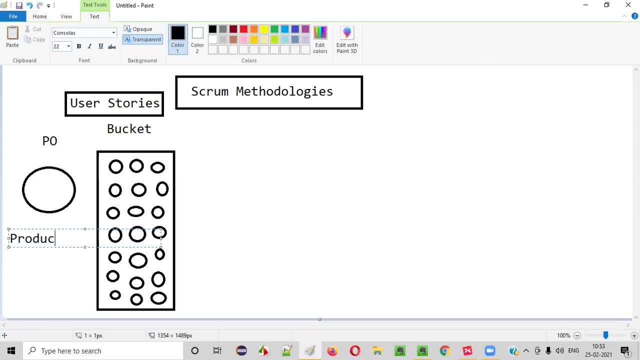 PO means product owner, guys. PO means product owner. Product owner who has a complete knowledge about the application and who knows the complete functionality and business of the application right. He will break the requirements that are required for developing the software into smaller chunks. 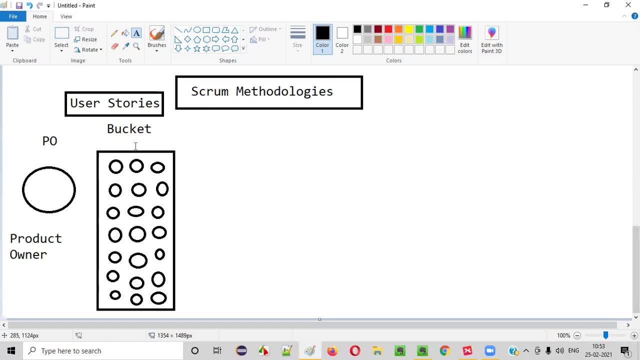 and put into the bucket And later what he does in this bucket. he will provide the priorities: okay, The first priority. second priority. okay, This one to be third priority, this one. fourth priority: okay, This one. some fifth priority, this one. sixth. 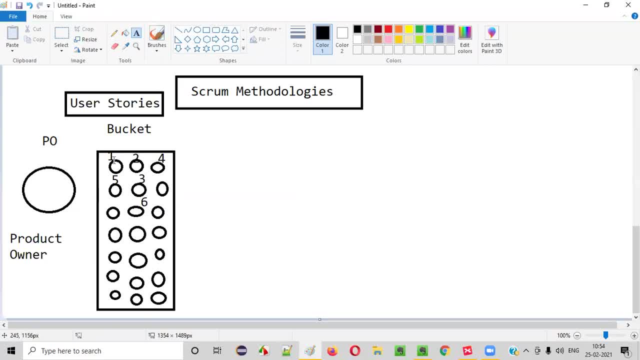 Like that, he will give the priorities: okay, Which one need, Which one need, Which one need, Which requirement need to be developed first? Based on that, the product owner will prioritize. prioritize the user stories, The product owner, based on the requirements that need to be developed first. based on: 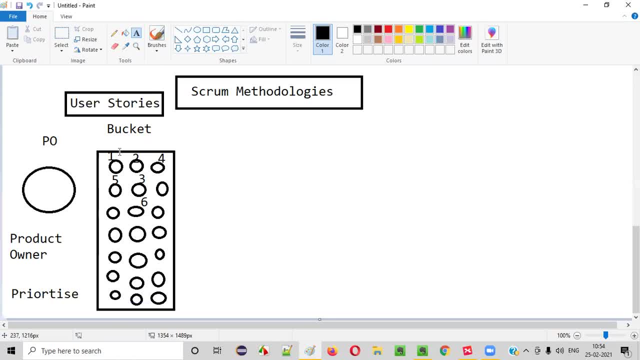 that kind of thing. he will prioritize the requirements like this. okay, For each and every user story here will be prioritized. This particular user story having some portion of the requirement for the development of the software is prioritized as a first priority. 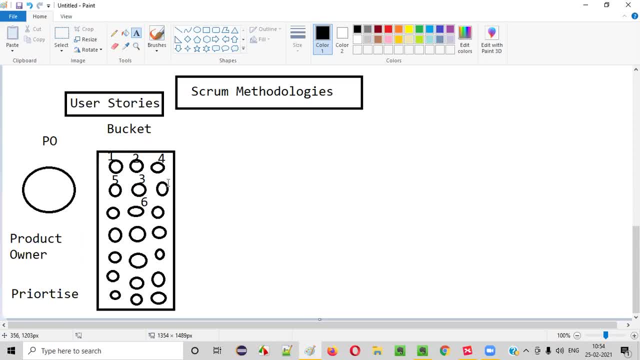 This one need to be developed first, like that. Fine, So after he prioritized all the requirements, that is, user stories in this bucket, okay, What this product owner will do is he will create something known as sprint. He will create something known as sprint guys. 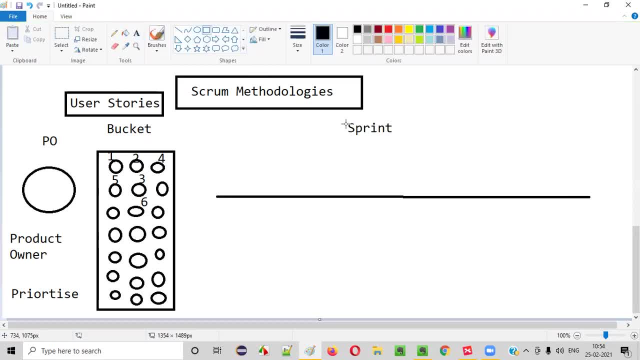 What is sprint? Okay, What is sprint? He will create something known as sprint. So what is sprint? Sprint is generally so. all the most of the projects follow the sprint in terms of four weeks to four weeks, to two weeks to four weeks. okay, 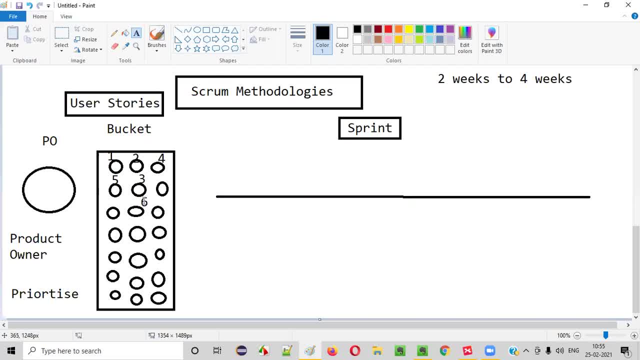 Two weeks to four weeks. This is the general duration of the sprint guys. So this product owner will create a sprint guys that will generally last for two weeks to four weeks. Let's assume that in this case, in this example, whatever I'm explaining, let's say the sprint. 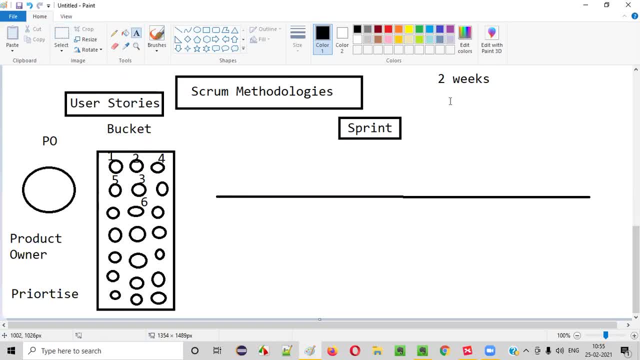 size or duration. okay, The sprint duration is. duration of the sprint is two weeks only. Let's assume that. okay, Most of the projects follow two weeks duration, guys. So now, this is a starting point of the sprint. 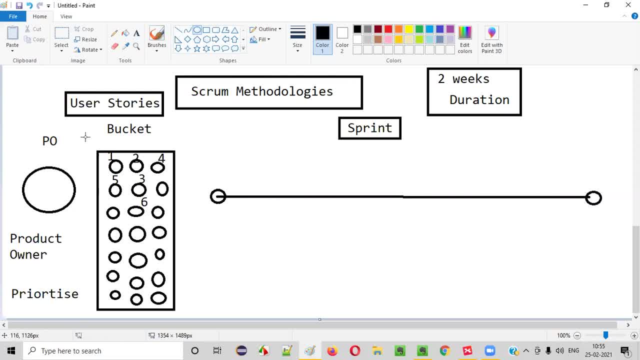 This is the ending point of the sprint. When the product owner creates this particular sprint, what he does is according to the prioritized. according he will actually take the prioritized user stories. okay, The high priority user stories, Let's say here one, two, three, four, five, six. 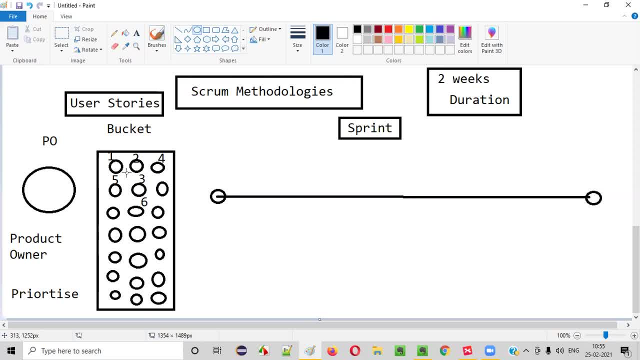 Six stories are there. Out of all the remaining stories, these first six stories are high priority, right, Those, those six stories he will add to the sprint. Okay, For this particular sprint. what is the duration of the sprint? Two weeks. 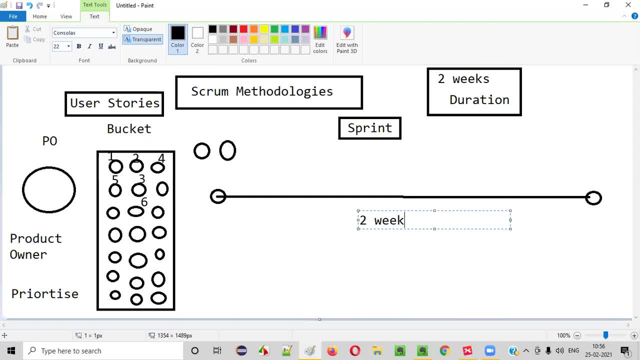 For this two-week sprint sprint can be four weeks also, guys, and here I'm taking example of two weeks. Here for this sprint, he is adding only a set of user stories according to the priority, That is, from one to. let's say, this story is prioritized as one, this is two, this is. 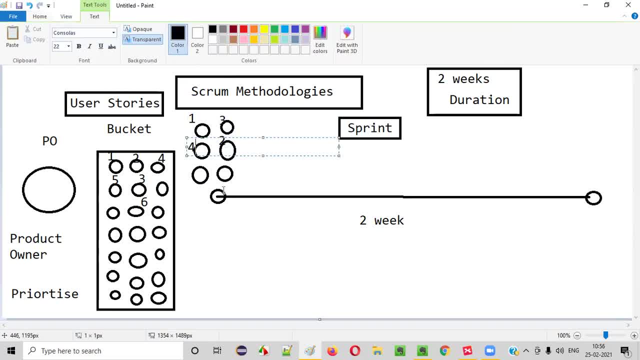 three. okay, He collected a few stories. only the requirements that he thought like. only this set of requirements he thought like this set of requirements. Okay, The requirements he thought like that they can be completed in two weeks, guys, okay. 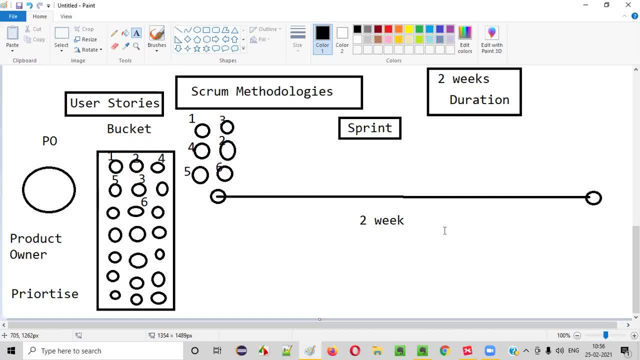 That requirements that user stories- high prioritized user stories- will be added into the first sprint. This is sprint one, guys. You can say this is sprint one, first sprint. So here, once the user stories are added here, what happens next is the development team. 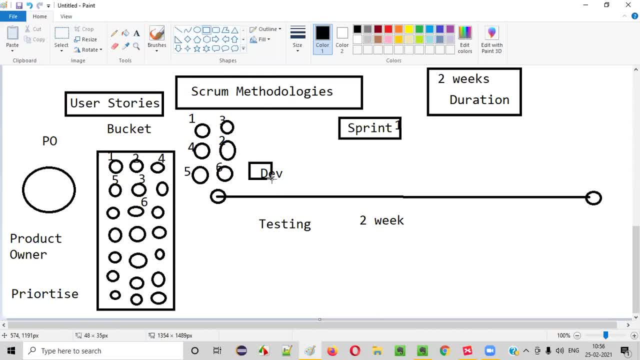 the testing team. Okay, There will be the developers and testers- right, These both people, okay, Apart from developers and testers. there will be some developers and testers. Okay, There will be some BA also. okay, Business analyst kind of people also. 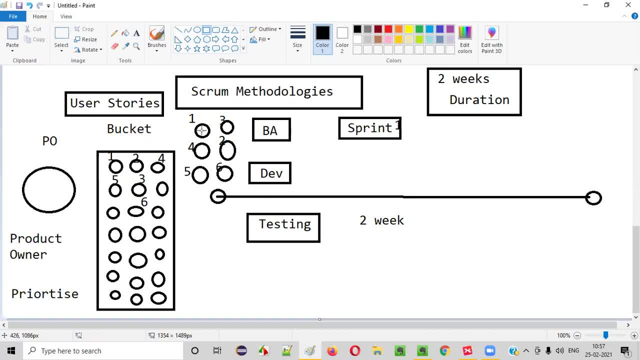 These business analyst people. what they will do is: okay, they will be writing the, they will be creating the user stories, guys. I mean, they will be describing the stories, How they will be described. let me show you one example. 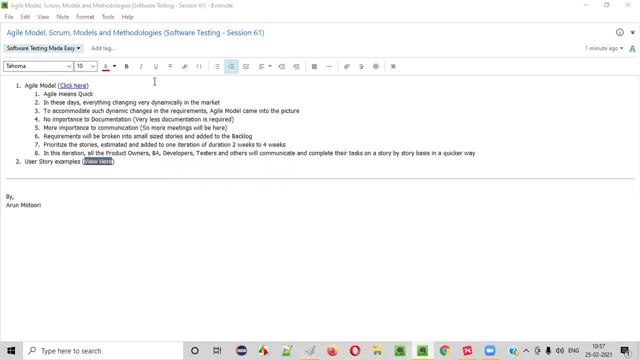 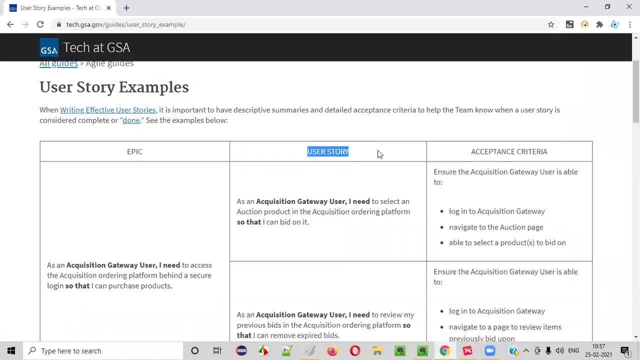 This is how they will be describing the user story. If you go and search here, there are some examples of the user stories provided here. guys, You see This is the user story For one of the examples of the user story. this is the user story. 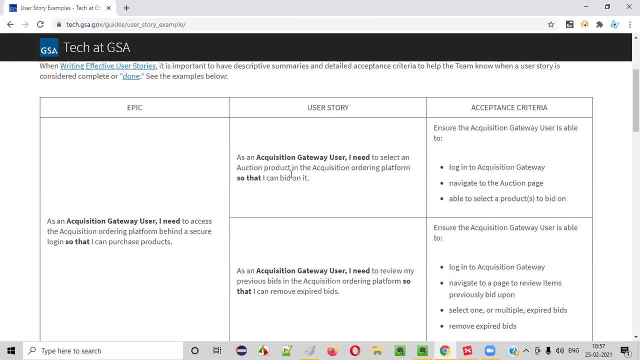 As an acquisition gateway user, I need to select- this is a title kind of story. okay, This is the title of the story For one of the stories. this is the title, kind of okay. As an acquisition gateway user, I need to select an auction okay. 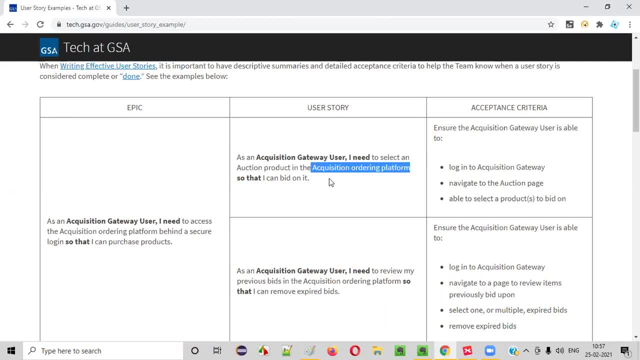 Product in the acquisition ordering platform In that particular software, we need to select an auction. That functionality is required. okay, These are requirement guys. Here. this particular line is explaining about the product. This is explaining about the requirement. what exactly is required as part of this user. 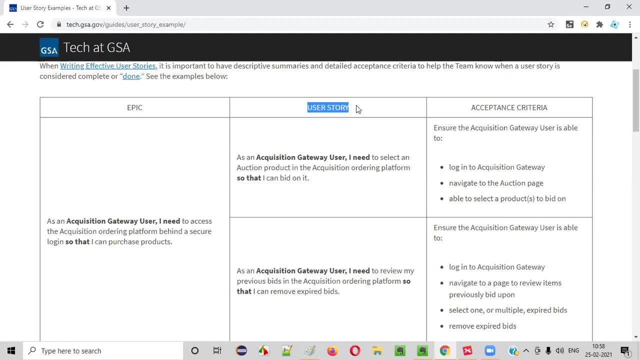 story- User story- is a small chunk of the complete requirements. right, That is nothing but a small requirement, breakable requirement, kind of thing. okay, So here, who will be writing this line, this particular line about that particular story? describing the story. 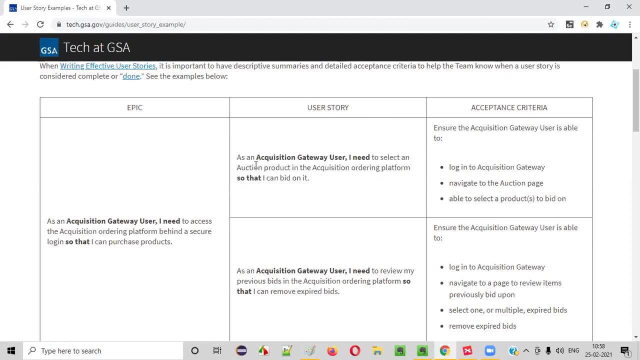 Who will be writing this line? Business analyst will be writing guys. okay, He will be writing. either business analyst or product owner in combination. they will be writing initially, But this line will be definitely written. Okay, This is written by business analyst. 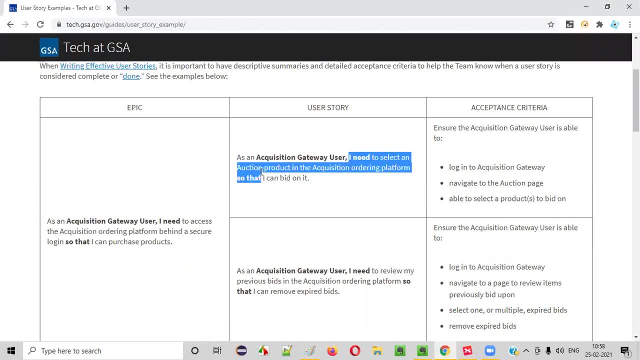 As an acquisition gateway user, I need to select an auction product From the software. we'll be able to select some auction product so that people can bid it. That is a requirement, And also business analyst will also. okay, business or business analyst will also do. 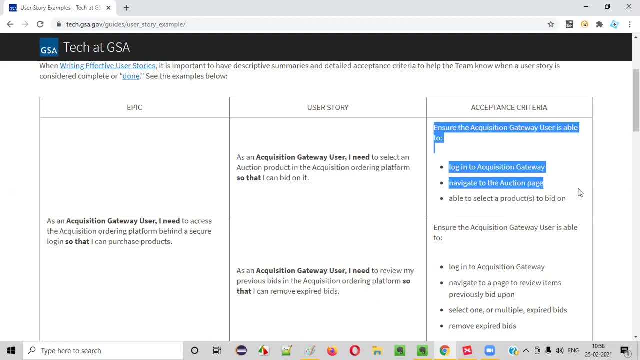 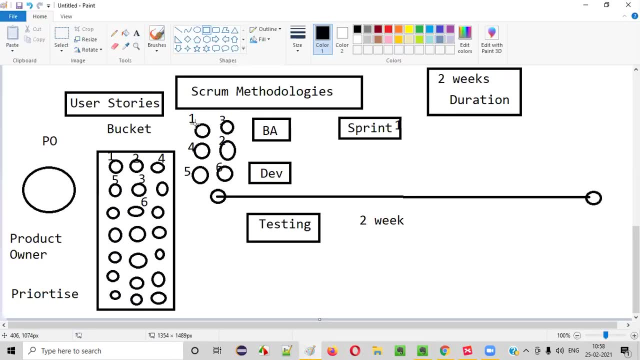 what They will describe this line, guys- They will describe this line in a better way- like this is acceptance criteria. they will call So here in this diagram, for each and every user story. that is one to three. Okay, 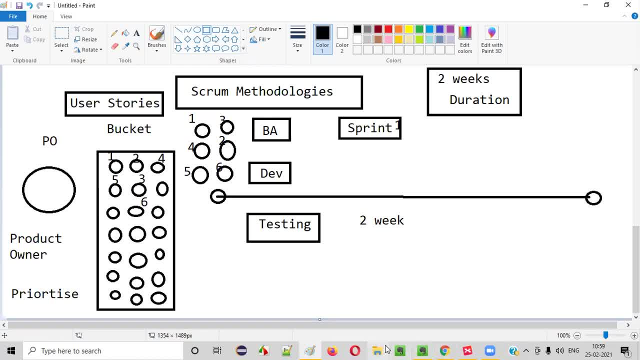 One, two, three, four, five, six, provided right For each and every user story. these two things will be available, guys, That is user story, and in that user story itself they will provide acceptance criteria. If I take this one, okay, the first user story, let's say this is a user story. 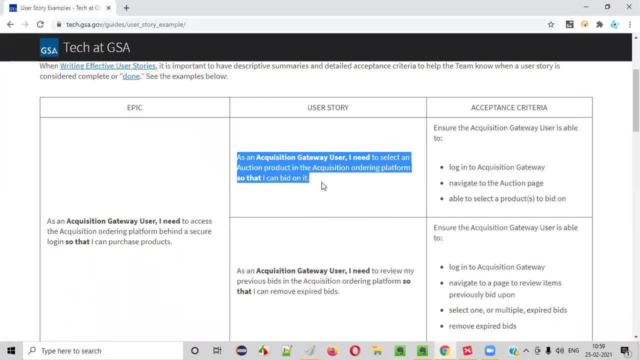 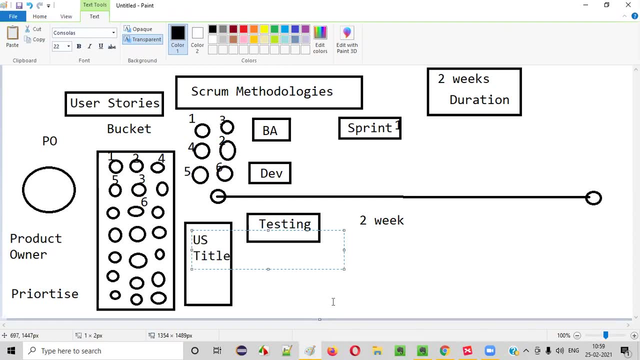 In this user story. this line will be there first. okay, as an acquisition gateway, This user story title will be there: user story title. After that, what will be there in the same, in this number one user story, or something? 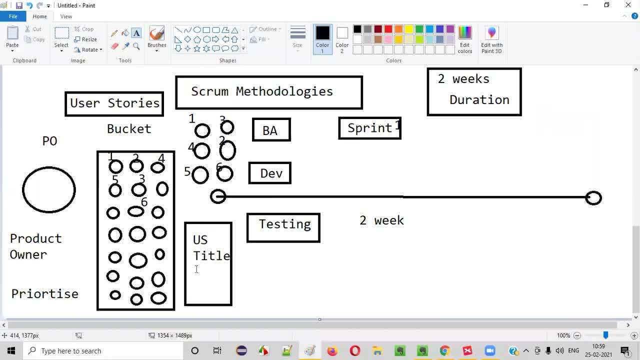 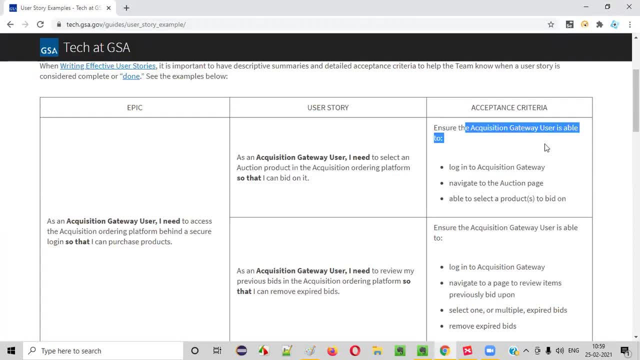 There will be acceptance criteria. okay, acceptance criteria- written. also ensure that acquisition gateway user is able to log into the acquisition gateway. navigate to the auction page, able to select a product to bid on. okay, Ensure the acquisition gateway user is able to log into the acquisition gateway. log into. 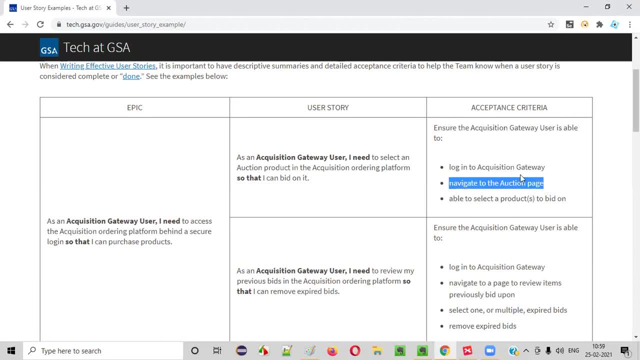 the software navigate. in the software we should be able to navigate to this auction page. In that auction page, the user should be able to select a product so that he can bid. okay, He can bid a product. Auctioning means you have to bid, right. 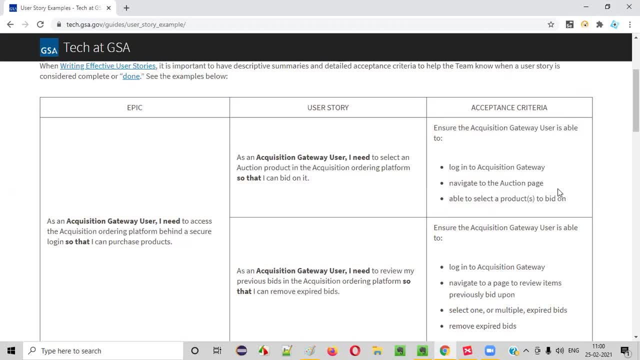 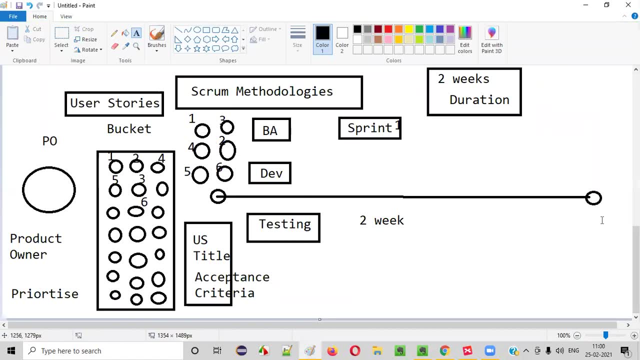 So you see, this is the title kind of thing, this is the description kind of thing. Description of the user story is nothing but the acceptance criteria. This thing will be clearly created by the BA guys Once the stories are added to the sprint. like this, BA will provide this proper title and 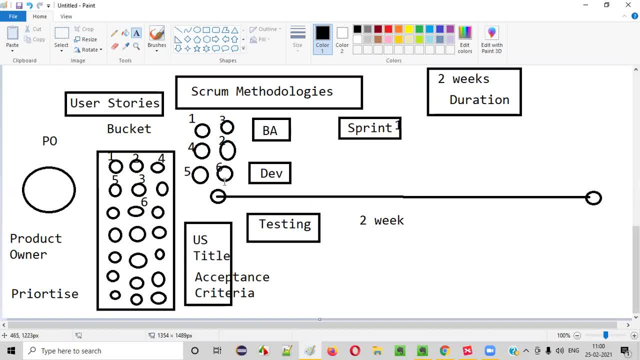 a proper need and proper requirement and proper acceptance criteria. Then what developers and testers will do After the BA is done, After the BA is completed, they will discuss all the review for the users. Then developers will, on the other team will basically discuss this data of the user苦. 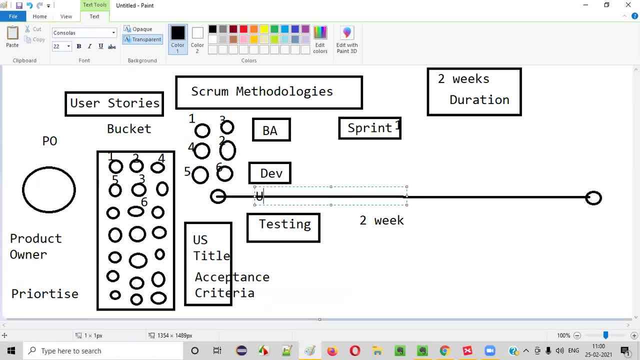 that we have written here. Okay, Before the, you will be sourced. the results of the search with the user story will be especially clear and clear. Then what the users usually will do Is because, uh, the desenvolpers and teachers areeightight, his authority they have to create. 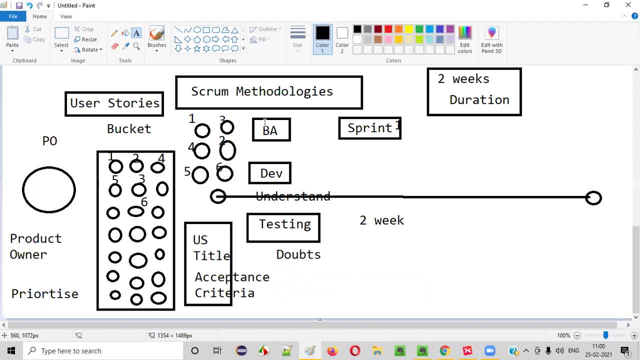 right, they will get doubts. these doubts will be asked to the, the people who has written this user story. business who has written the user stories. right, they will ask the doubts. business will clarify the doubts. okay, business will clarify the doubts later. what will happen after the business? 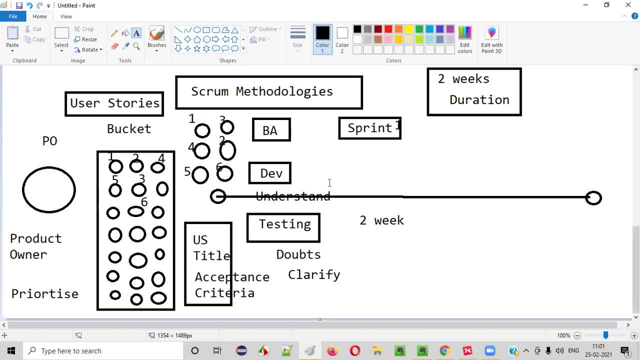 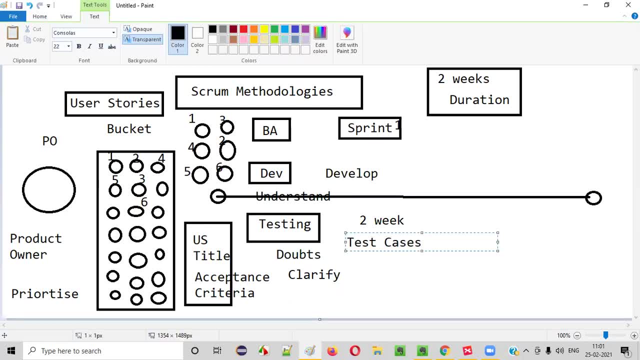 has clarified the doubts. okay, then developers and testers will do their job. developers will do what guys? they will develop. testers will do what guys? they will start writing the test cases, test scenarios, whatever that is required. okay, and they will attach. okay, if they here, testers are not. 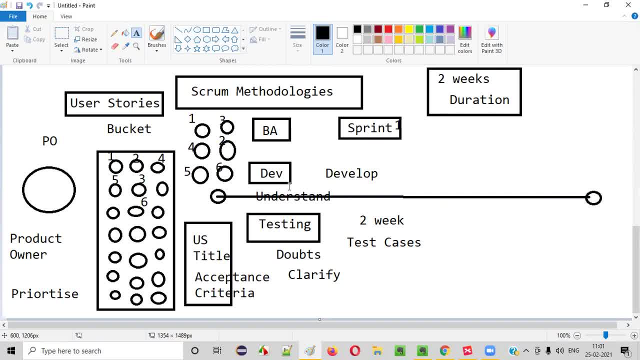 creating the test cases for the entire entire application. they will only create the test cases for this particular requirement that is specified in this only user story. in this particular single user story only they will write the test cases. they are not going to write the test cases or test. 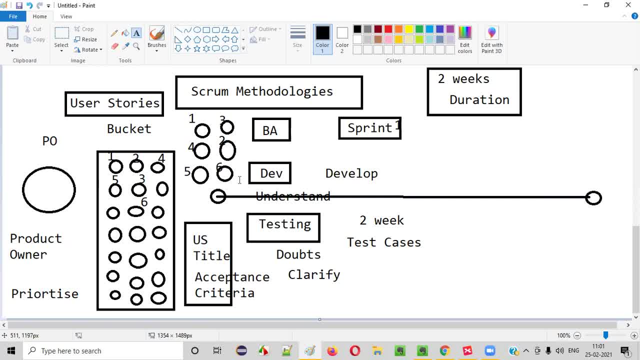 or scenarios are for the complete, complete application here, only for this requirement they will write the test cases. developers will also not develop the complete application. they will only focus on this requirement and develop that particular requirement only so. but what is the goal of this sprint, guys here? the goal of this sprint is to complete the 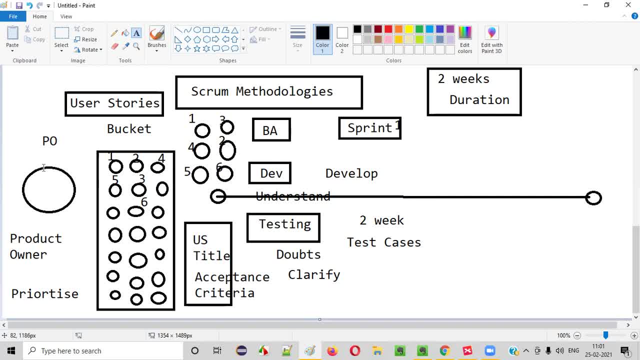 development and testing of this particular requirements assigned by this product owner to this particular sprint, by the end of the sprint, all these five to all the six stories. okay, here, for example, here we took six stories- all the six stories need to be developed and fixed. uh, developed and tested by the, tested by the team. here team is development. 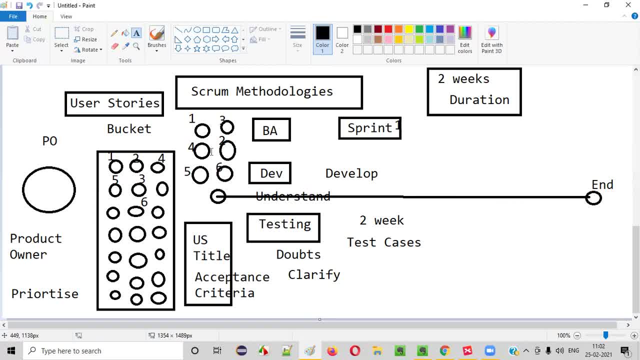 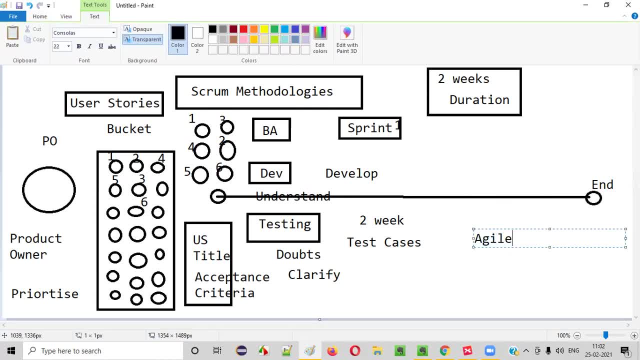 team and testing team. so are there any other team members in this, uh, agile scrum? generally? yes, guys, there are more people also, okay, who are agile team. actually, who will be there in agile guys? as i already explained, product owner will be there. okay, who is in charge? or in the beginning he came right. uh, who is who knows everything about the? 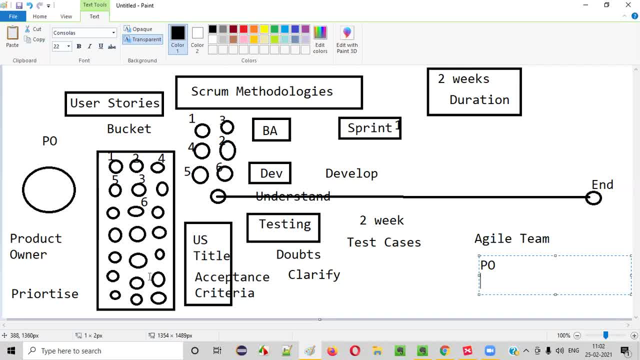 application. who has a complete knowledge? who will be creating the user stories at a high level and then prioritizing them as into the student? okay, his role is like that: after product owner, we have uh, home guys. okay, we have the business analyst- is there? okay, who will be describing these user? 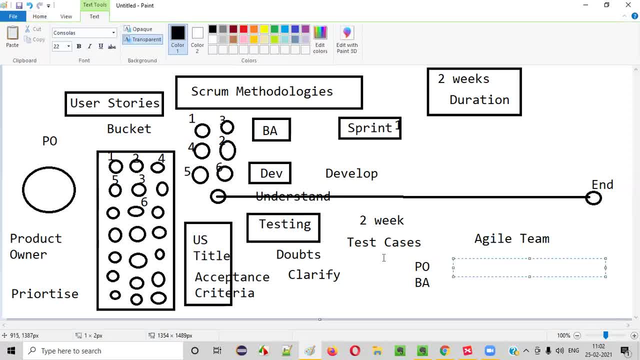 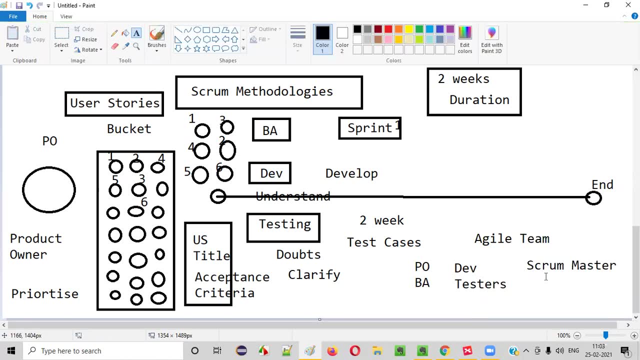 stories. then, uh, we have other people also here. already. we covered developers and testers. right, divine testing team is covered. developer center testers are there? apart from this, developers and testers, there will be scrum master- this, okay, there will be scrum master. this scrum master, okay. this scrum master is in charge. 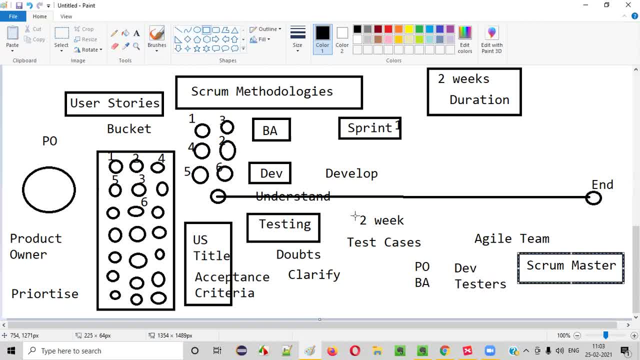 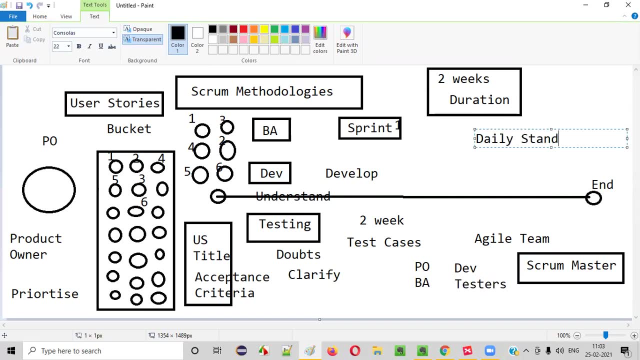 okay, this scrum master is in charge of this complete delivery of the requirements. okay, he will take care of whether the things are going fine or not. so what the scrum master will do, he will schedule daily stand-up. okay, he will. he will take care of the daily stand-up meetings. so everyone in the 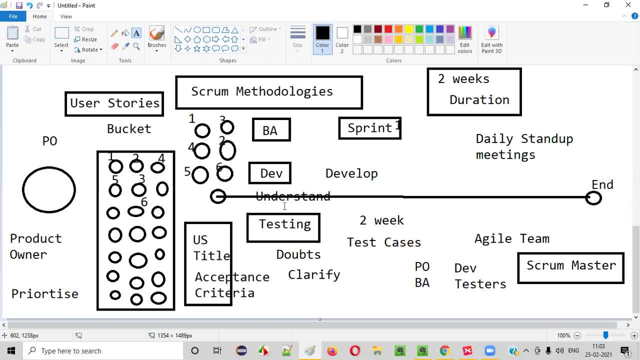 team like developers business- i mean developers, cba is their ba- and testers and any other people in the team will be attending this daily stand-up meetings and owner for that meetings is scrum master. scrum master is a owner who will be leading that meetings. he'll be like there the discussions. 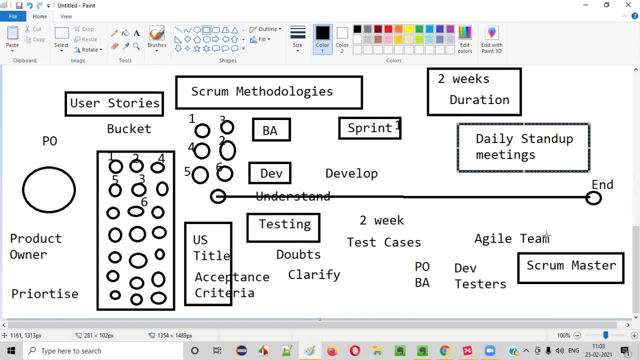 will go on like: what is the progress? what we completed? what development team completed? what testing team completed? are there any blockers? all those things will be discussed in the daily stand-up meetings. okay, who will be taking care of that? scrum master? okay, scrum master takes the ownership for completing the task. guys, okay, if? 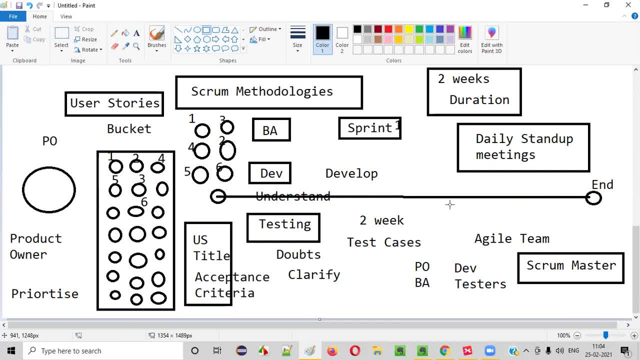 something is not going well, he need to solve the problem why. it's why some blocks are coming. so what need to be done? so is there any client communication missing? he will take care of that. guys, if the process is not going well, scrum master is the one who will take care of the things. 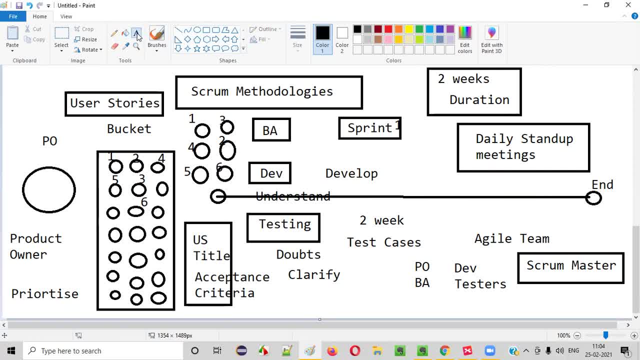 fine, daily stand-up meetings and also guys at the end of every sprint. some meeting will be conducted like retrospective meeting- okay, retrospective meeting- where everyone in the project will be there and they will be discussing what went correctly, what went wrong- okay, what can be improved for the next sprint. 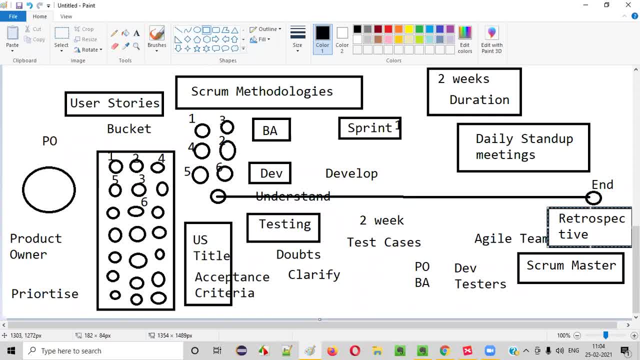 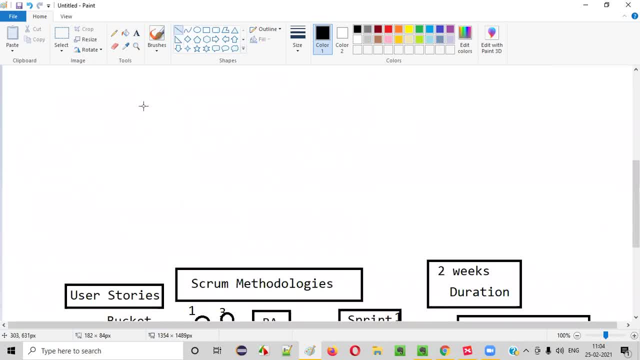 okay, let's say these six stories got successfully developed and tested by the uh, tested by the team and completed by the end of the sprint. then what will happen, guys? next sprint will start. second sprint, sprint to two, will start. same two weeks timeline. okay, sprint two will start after. 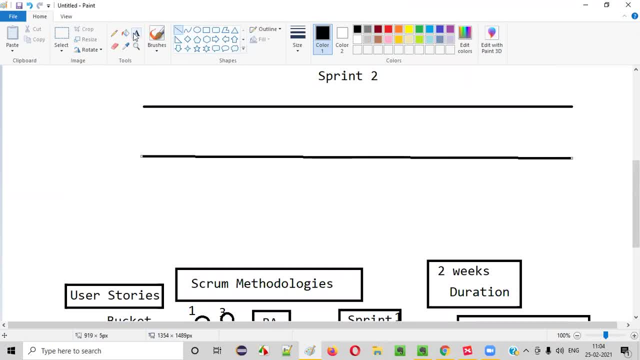 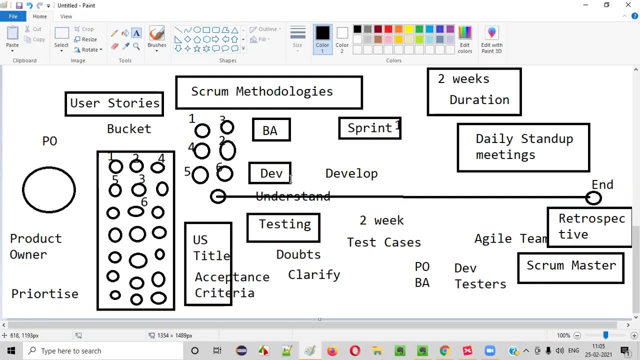 the sprint two is also completed, then sprint three will start. what is the advantage here, guys? what is the advantage of the sprints? because of this models? there are a lot of advantages coming in, guys. okay, because of this, uh, following this agile scrum methodology- right, there are a lot of advantages. 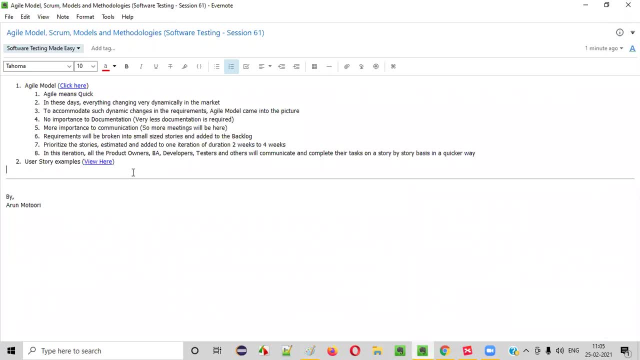 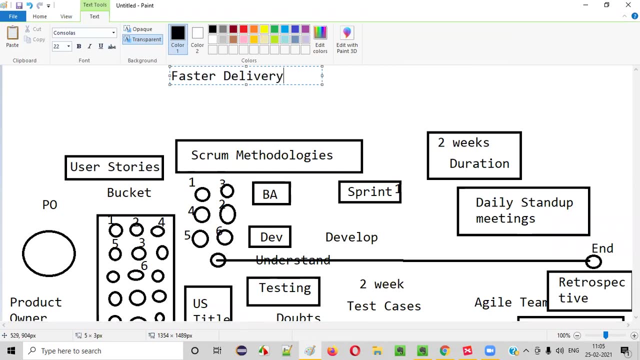 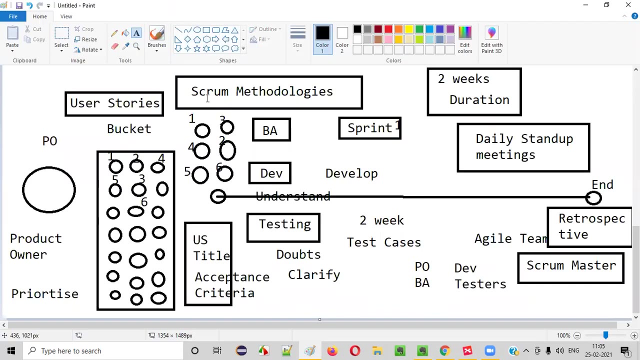 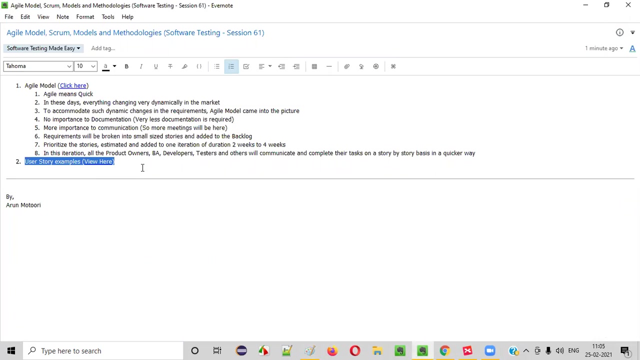 guys. so the advantages here are okay. the advantages here are faster delivery guys. faster, okay, faster delivery. software will be developed faster and delivered faster guys. because of this model, okay, because of this agile model and agile scrum methodology right, which is famously used in nowadays in the project right, projects are delivered, developed and softwares 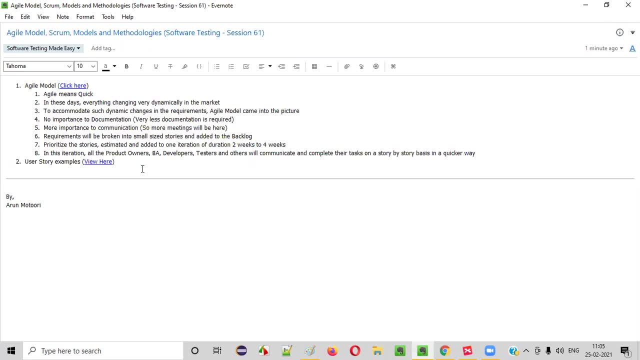 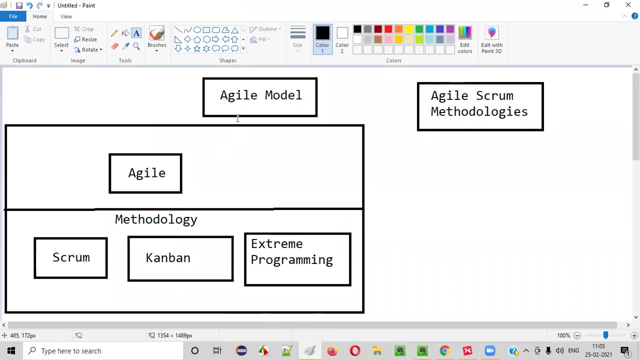 are developed faster and projects are delivered faster. okay, that is the advantage. so now let's understand what is agile case, after you understood all these uh things about the agile right, agile model, uh, sdlc model in that methodologies, then we have the best practices, like practices of the gel. 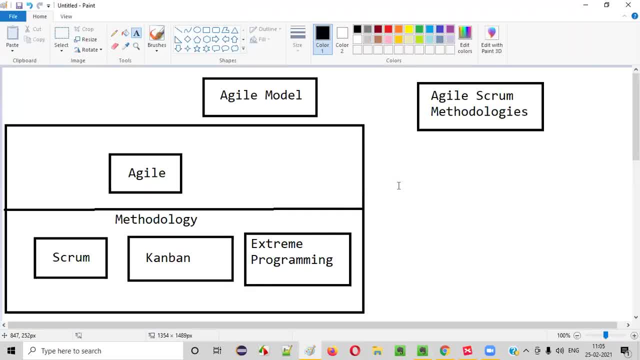 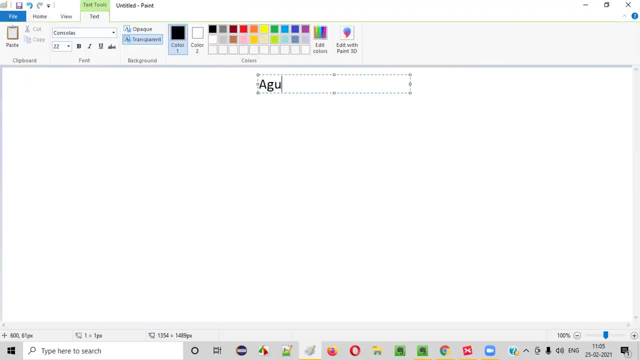 then i explained about one of the methodology of the agile. now you understood what exactly agile at a high level right now, what? why agile then? why everyone is using agile. then what is the benefit of agile? how, uh, how, how it is benefiting everyone in the software development and releasing and etc. 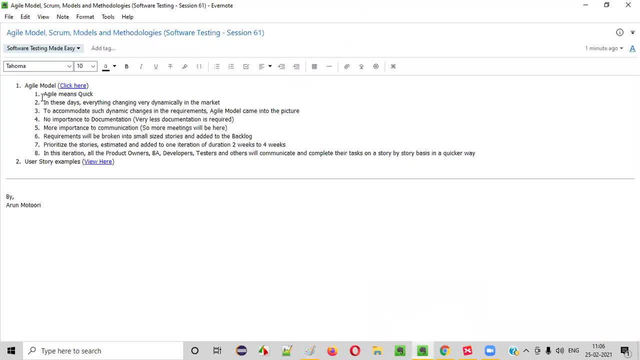 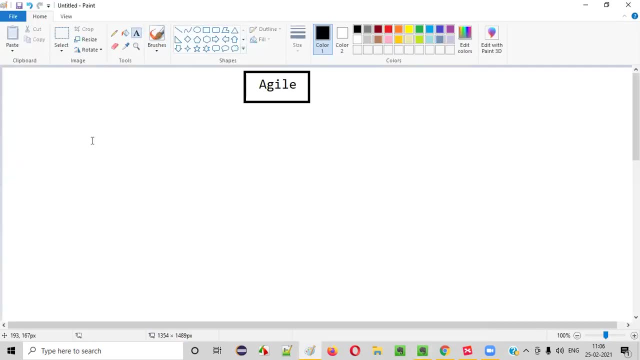 okay how this model is uh helping so in agile guys, what's actually happening here is so nowadays, right, nowadays, uh competition is very high guys. okay, competition is very high if you take any uh popular applications like flipkart or amazon. okay, if you take any popular applications like flipkart or amazon. 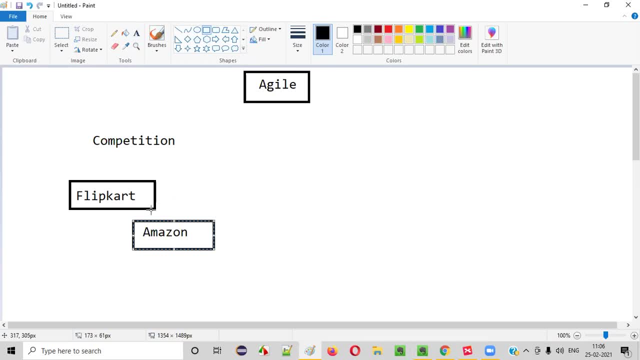 so what's happening in this flipkart and amazon guys? every day some new functionalities are getting added. okay, they are competing with each other. flipkart- amazon are competing with each other and one day the amazon comes up with one feature, flipkart will come up with another. 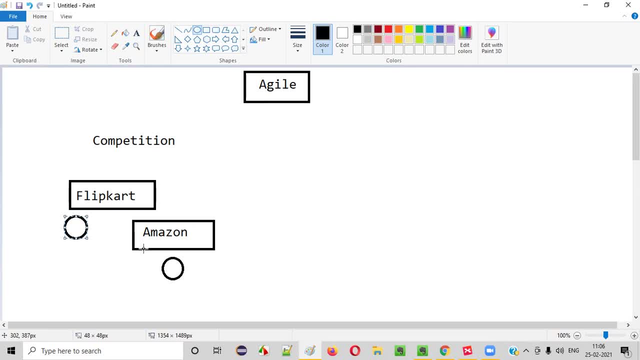 feature: okay, as a competition, they want to head be head in the market and make the delivery of the products uh, easy for the customers. okay, they will make cash on delivery. a lot of things one day. delivery: okay, you will get the amazon prime subscription. how these functionalities are. 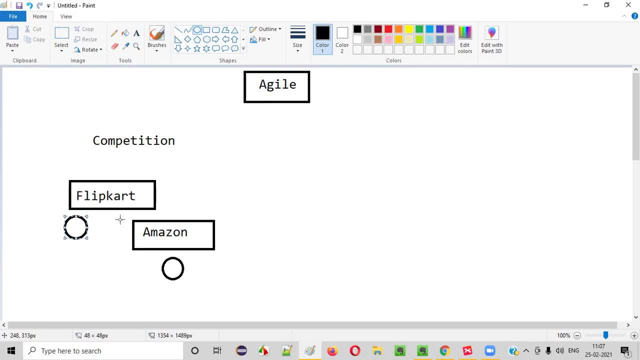 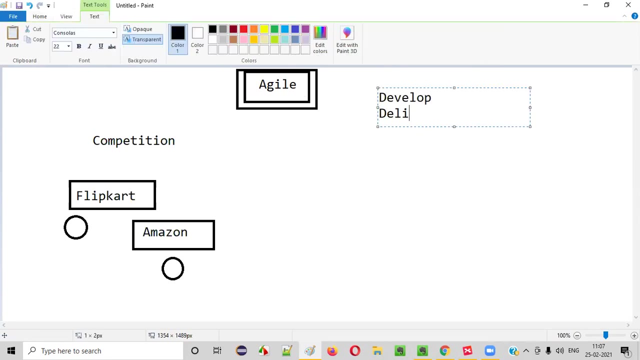 coming. they are competing with each other, they have their own marketing strategies and for for such kind of highly competitive applications, agile is about best model guys- okay, best sdlc model, software development, lifecycle model. because using agile we can develop, develop and deliver the software or functionalities. software functionalities in. 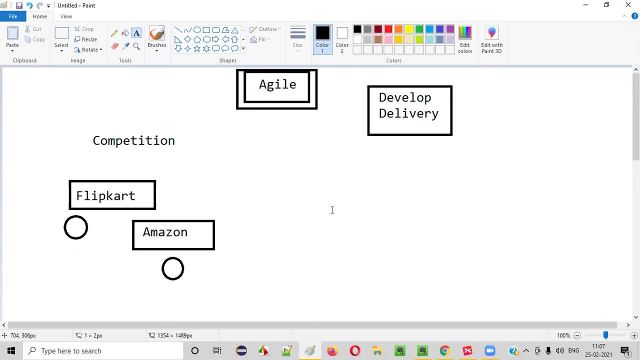 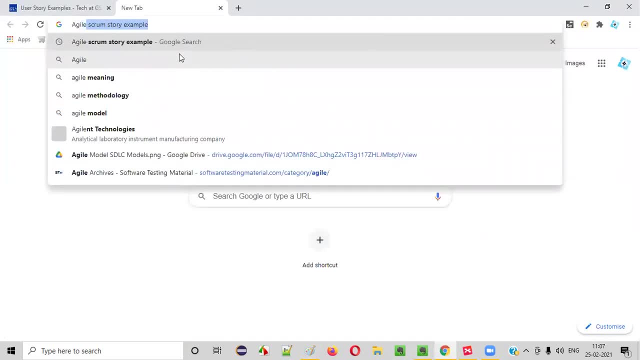 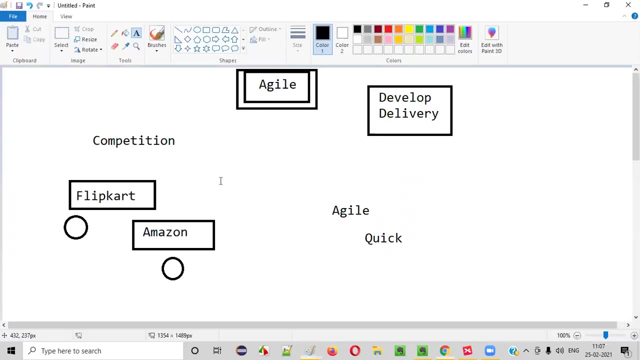 a faster way. the meaning of the agile itself is: quick guys. okay. the meaning of agile itself is: quick, the faster. okay, let me type in the google. you will understand if i search for agile here. the meaning of agile is: agile means able to move quickly and easily, so fast. 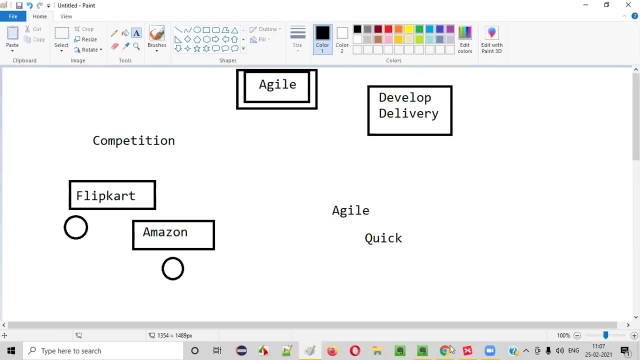 early. okay, firstly, you have to develop and deliver. that is agile guys now. so agile came into picture because, because of these competitors, competition getting increased in the market and companies are fighting behind each other by developing more new functionalities and marketing strategies are very rapid, fast, right to accommodate such kind of dynamic. 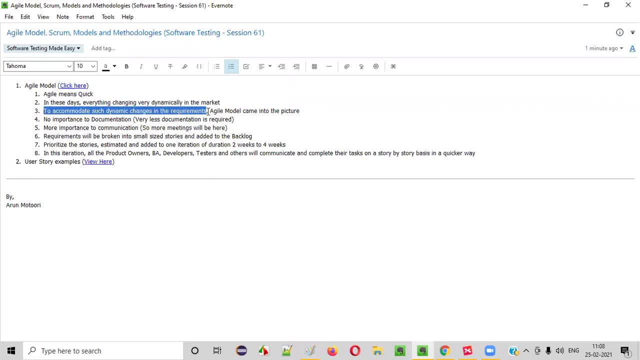 changes in the requirements. okay to accommodate such kind of competition where dynamic changes need to be implemented very fast and delivered into the market. right, and agile model came into picture. this is where the agile came into picture: guys and uh. here in agile there are few things followed, guys, uh, which makes the things more easier. and 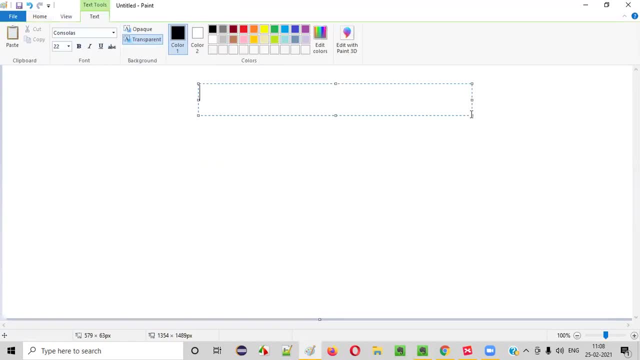 faster. okay, one thing about agile is here: less importance for documentation. guys, here you are giving less importance for documentation and more importance for communication. okay, in agile, this is the main line, guys: less importance for documentation and more importance for communication. traditional projects- what you will do, guys, where agile model? 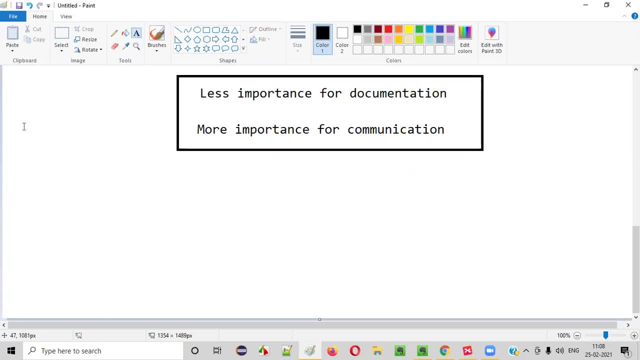 is not followed, you will firstly understand the complete requirements which are created and sent to you by the client in a separate brs srs documents and when, once you understand the complete requirements and ask the doubts and clear, then you will start the planning for the complete 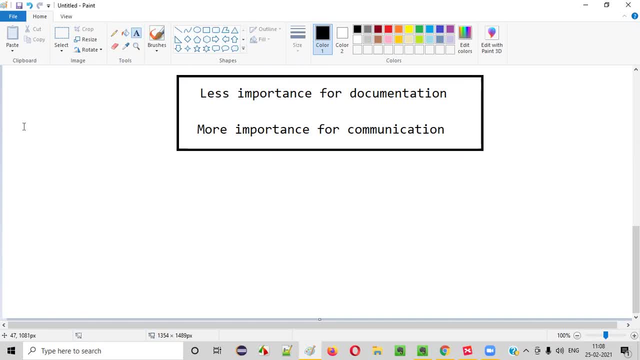 project. then you will do that uh. then you will write the complete test scenarios. then you will write the complete test cases documents. you'll you'll get it approved by the client or client poc, whether that uh written test cases are correct or not right. this is a very long process, guys. that takes a lot of time. that 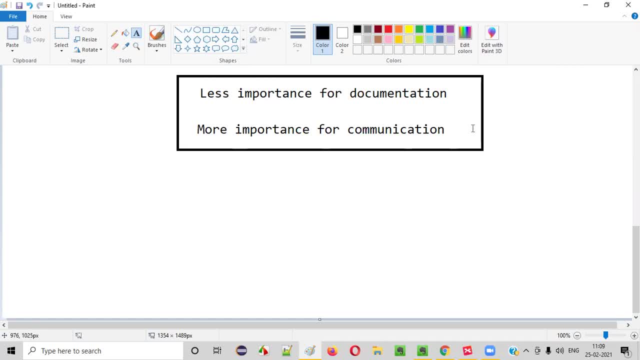 will waste a lot of time here. instead, less importance for documentation. you don't have to create some excel documents or some other documents or something here. simple, you will get a user story. for that user story only. you will work, guys, okay, you'll. you'll have a better focus. 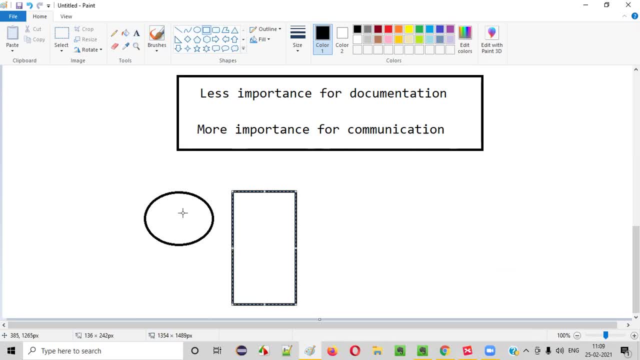 here. if i give you 100 requirements and ask you to work, you'll. will you have a proper focus, guys? you'll have less focus, but in agile, guys, since the requirements are properly break down instead of giving all the requirements for you at a time, in a sprint and 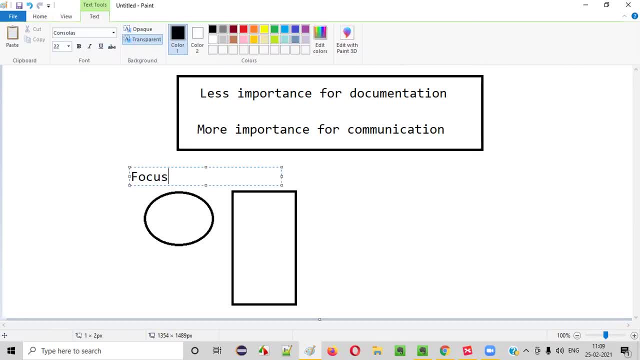 giving only six to ten requirements. is the focus increased or not? here we have a better focus. okay, in case of agile, we have a better focus because only few requirements are given. the doubts will be clarified fast here: more communication, more, a better review process, better feedback will be there and, uh, you don't have to document very lengthy documents here. less: 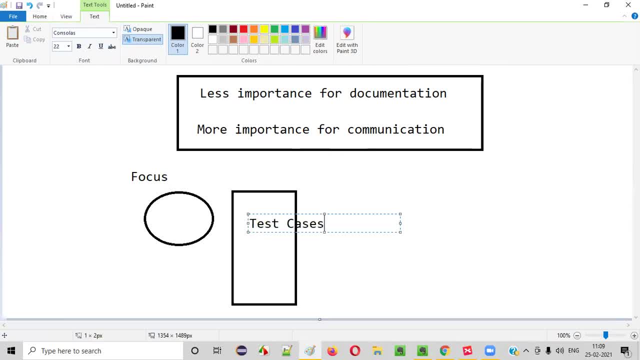 importance for documents where you'll simply creating some test cases in the same user story itself. okay, for the user story itself, where the title and description are provided, you will simply attach the test cases in the that particular chunk of requirement in the user story itself. that's why less importance for 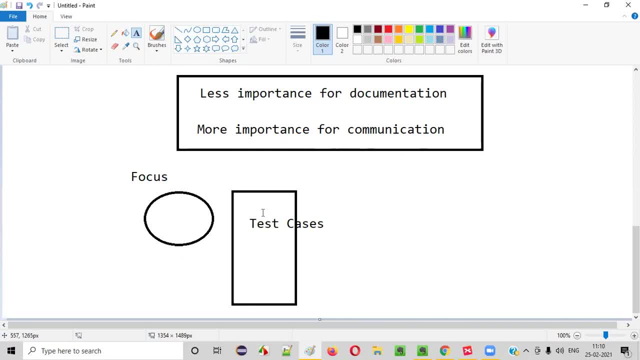 documentation and more importance for communication. here more thing happens about communication, guys. we we talk about requirements here here. uh, in the traditional process, the traditional, non uh like sdlc process, their requirements are very huge, guys. okay, requirements are very huge and, uh, the communication is, because of the less focus there, the communication won't happen in proper way. 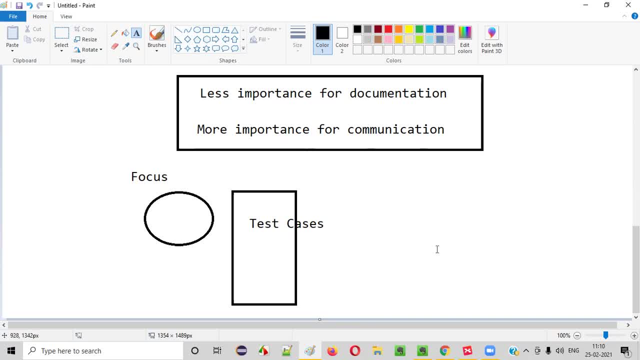 feedback also will not come in a proper way. if you write thousands of test cases and share with the client, the client will be able to review all the thousand test cases and feedback in a better way. no right, the focus is not there, but here the focus is better, to the point everyone will be. 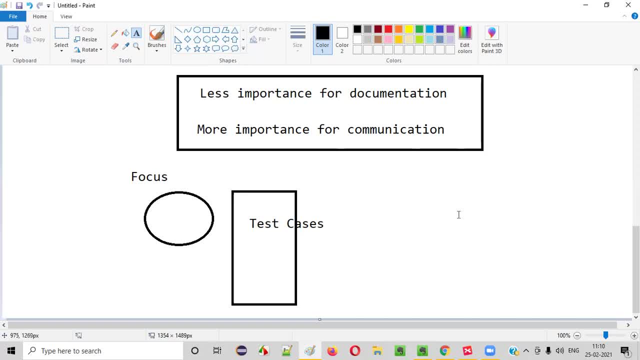 communicating. okay, even the developers testing team. everyone are working at the same level. developers will do some development while testers will working. they'll discuss the things. okay, everyone is communicating in the team guys. more importance is for communication. a lot of meetings will happen rather than uh, okay, rather than creating the documentation, he will meet importance. 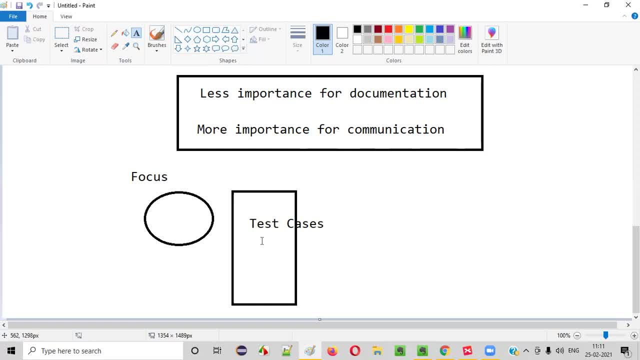 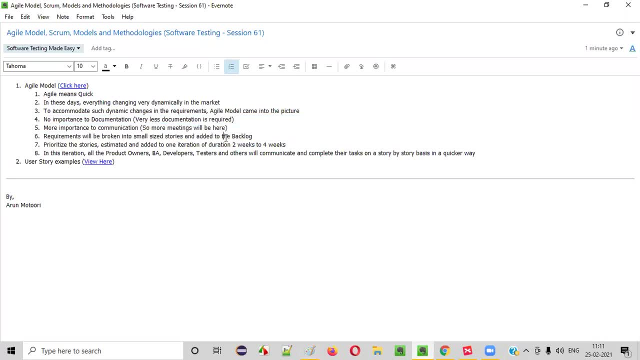 is given for meetings and communication and the kind of process that we are talking about and feedback and etc. will be more guys, okay, okay, so, so that's all about, uh, agile guys. okay, hope you understood what exactly is agile, right? agile is one of the popular sdlc models that are used by 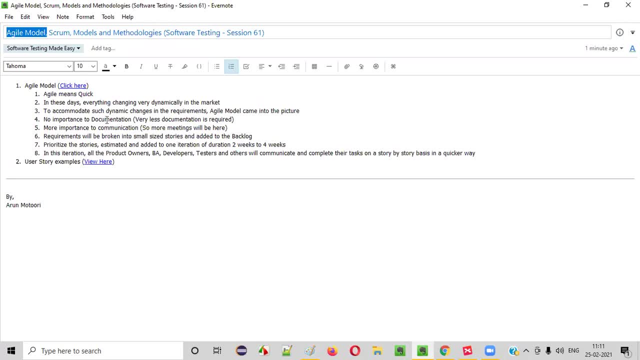 most of the projects nowadays, because it accommodates dynamic changes and where competition nowadays competition is very high, where dynamic changes happens like anything. because of that, this kind of models came into picture, and agile model is very successful and being used in the market right now also. okay, so so this is all. 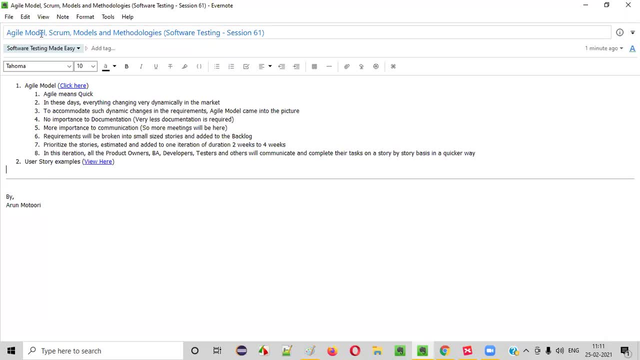 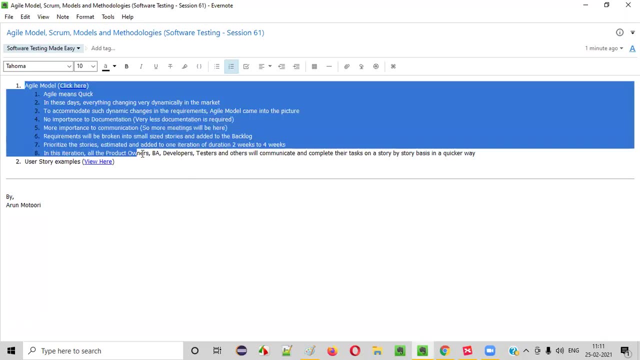 about agile sdlc model guys. i'll be explaining more about this- agile methodologies and best practices of the agile- in the upcoming sessions. okay, this is not the right time for now, if you understand this. whatever i explained in this session, that will be enough as part of the